In this tutorial, you're going to learn all about what chat GPT is, how it works and, most importantly, how you can use it to boost your productivity as a software developer. As a seasoned developer and teacher, let me tell you: chat GPT is a game changer you don't want to miss out on, Don't? 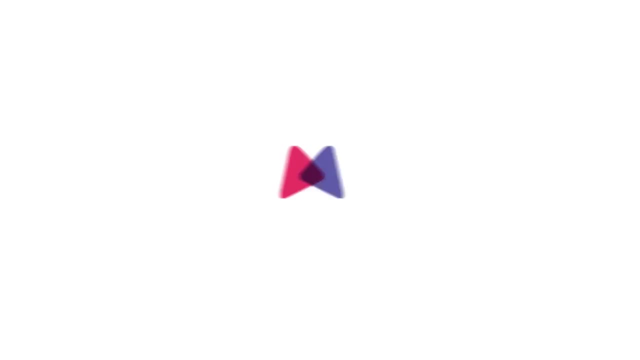 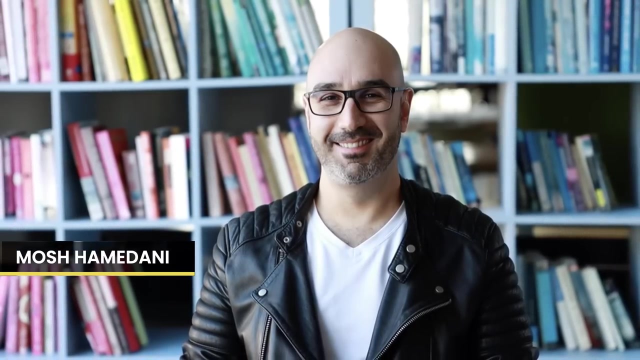 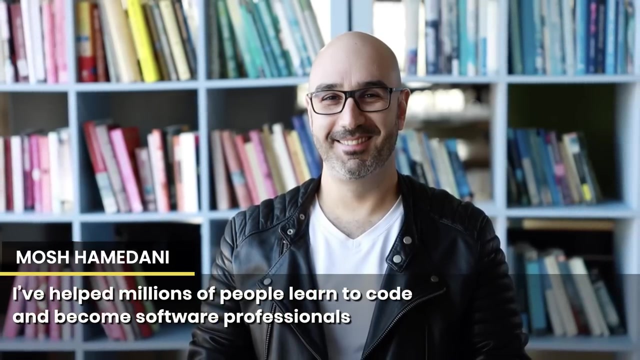 take my word for it. just watch this video and see for yourself. My name is Mosh Hamadani and I'm super excited to be bringing you this tutorial on chat GPT. I've helped millions of people learn to code and become professional software engineers through this channel and my online school. 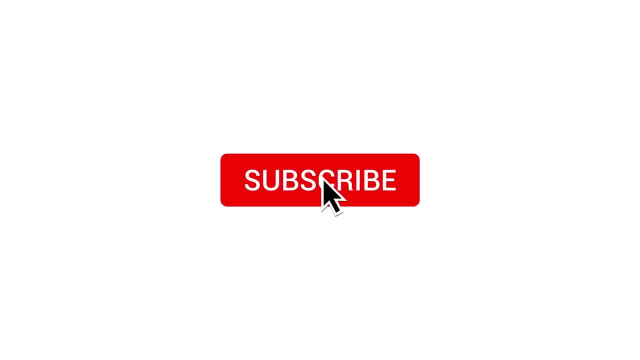 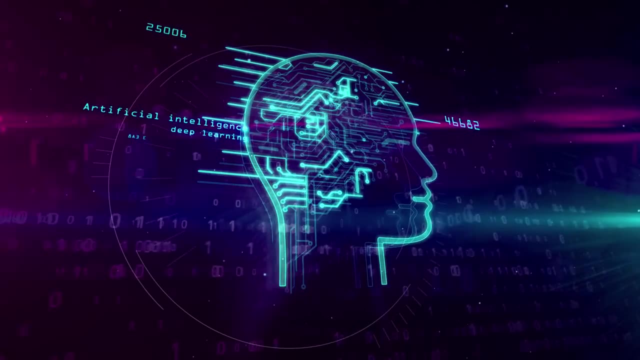 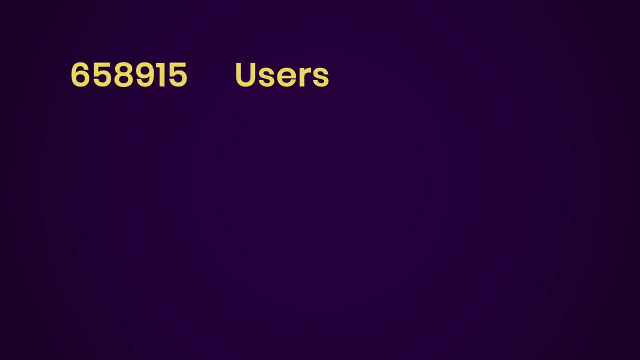 codewithmoshcom. If you're new here, make sure to subscribe so you never miss a video. So what exactly is chat GPT and how does it work? Chat GPT is a cutting-edge AI tool created by OpenAI. It was released in November 2022 and gained 1 million users in just 5 days. In comparison, 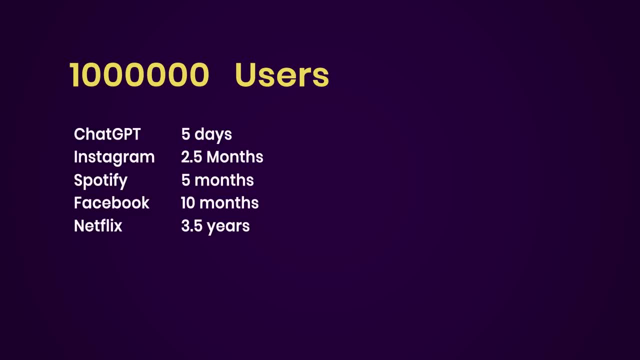 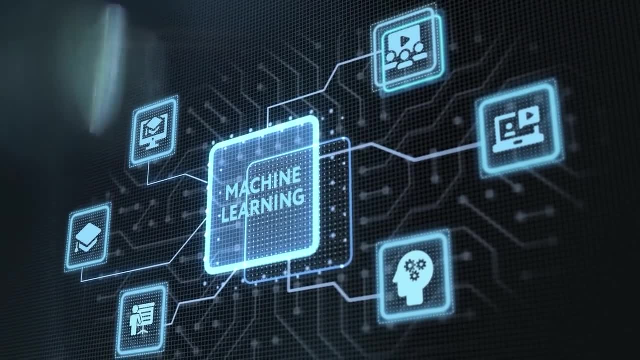 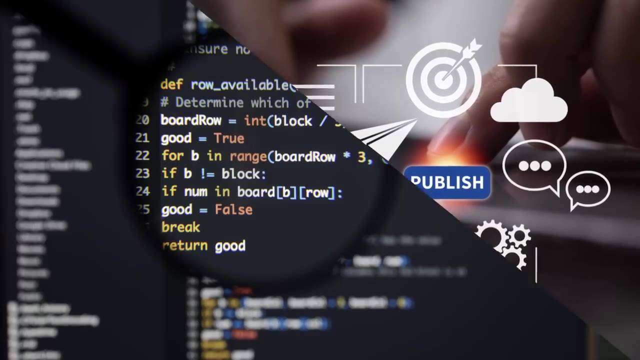 it took Netflix 3 and a half years and Instagram 2 and a half months to get the same number of users. Chat GPT is an advanced language model that can understand and generate text. You can use it to create content for your website: write articles, emails, tweets, cover letters and so on. You can. 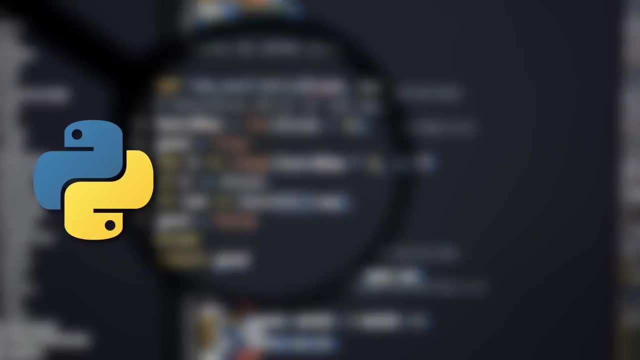 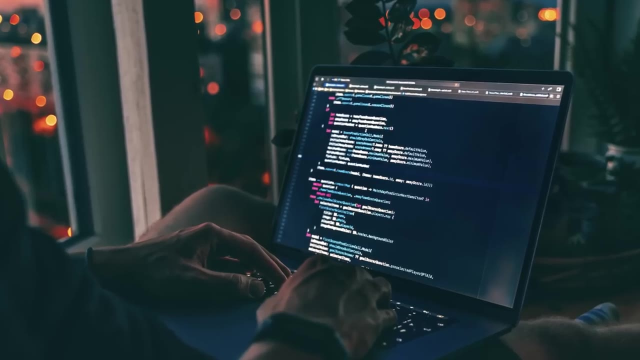 also use it to generate code in a number of different programming languages like Python, JavaScript, HTML, CSS and much, much more. You can use it to generate dummy data, write unit tests, translate text or code from one language to another. You can use it to explain code, For example, if there's a piece of 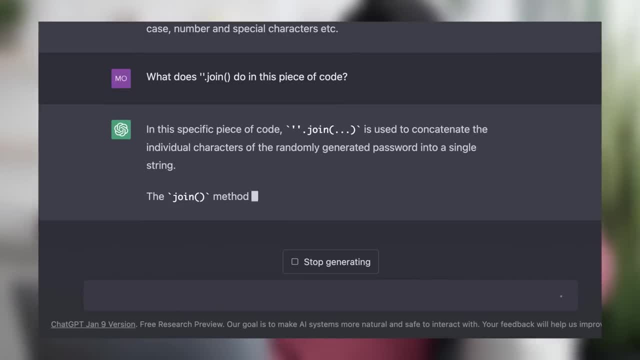 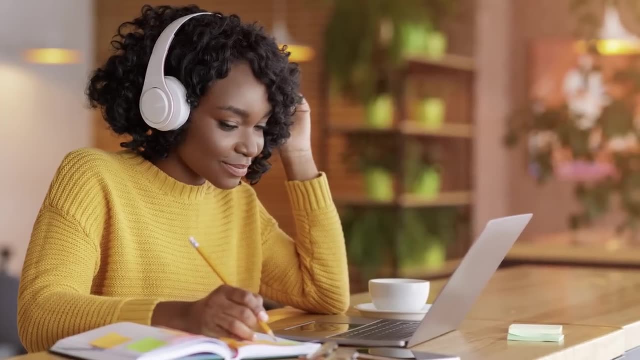 code you don't understand, you can ask it and it will explain to you like a patient teacher. But I have to be honest, sometimes it explains too much. Chat GPT can also help you learn and remember things faster. For example, you can give it some text and have it ask you a bunch of questions. 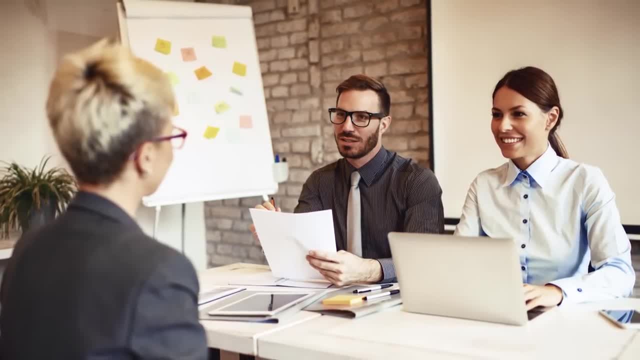 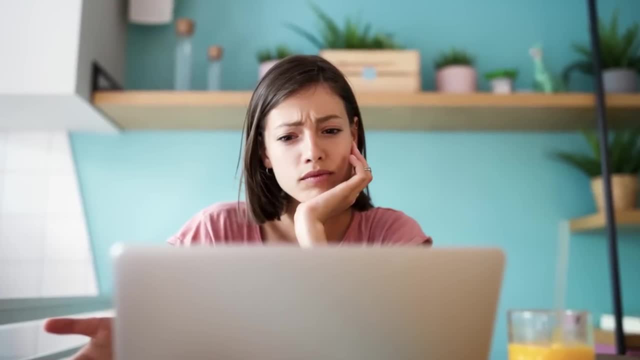 It can also prepare you for job interviews. You can have it improve your resume, write a cover letter for you and also interview you like an interviewer. Now, do you think Chat GPT is going to take your job? Let me know in the comments below. The reality is whether you. 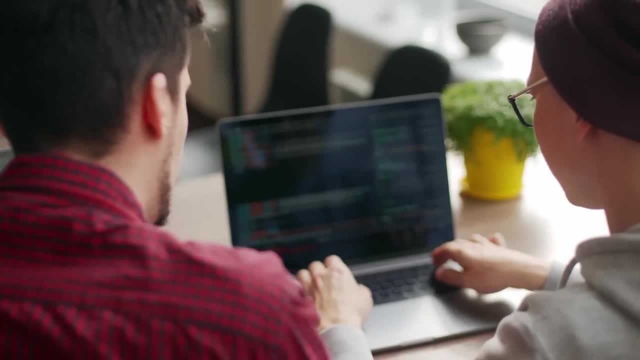 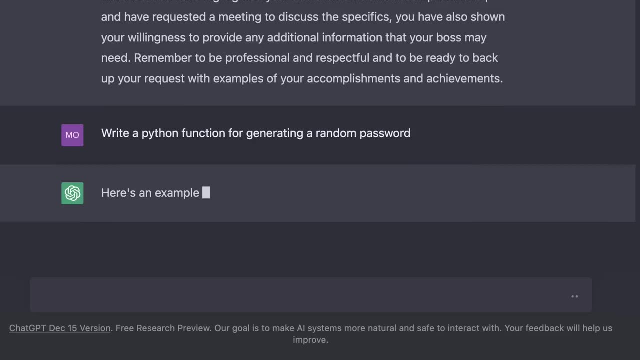 like it or not, Chat GPT is here to stay. In this tutorial, I'm going to show you how to use it to get more creative and get things done a lot faster. I'll be showing you various examples for different programming languages, both for beginners and experienced developers. But before we dive into 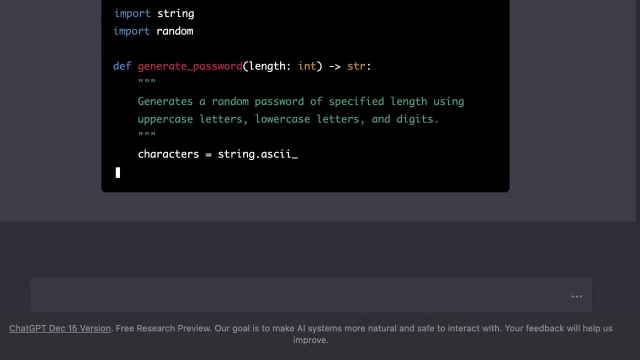 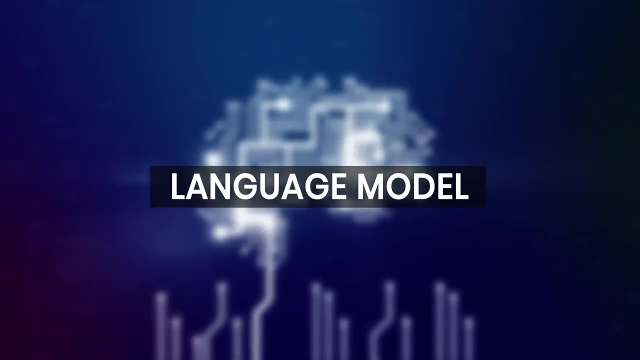 that let's take a moment and understand how Chat GPT works. Chat GPT uses a type of artificial intelligence called a language model. Chat GPT is a type of artificial intelligence called a language model. A language model is a type of software that is designed to understand and generate human. 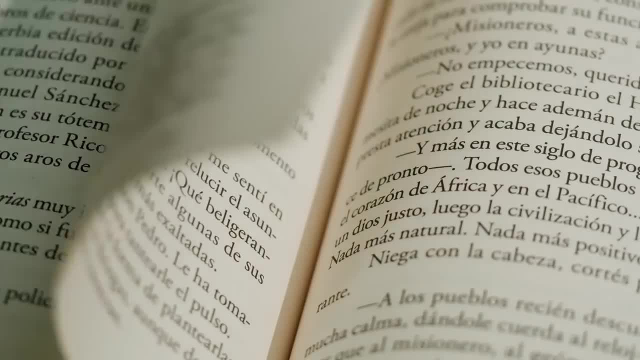 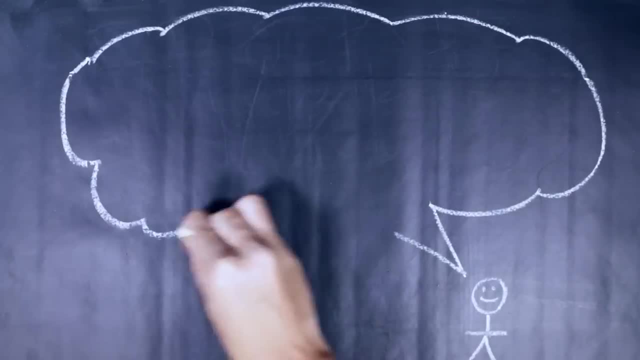 language. It does this by looking at a large amount of text data and learning the patterns and rules of a language. For example, if the language model is trained on a lot of English text, it will learn about the grammar and structure of English, as well as the meanings of words and 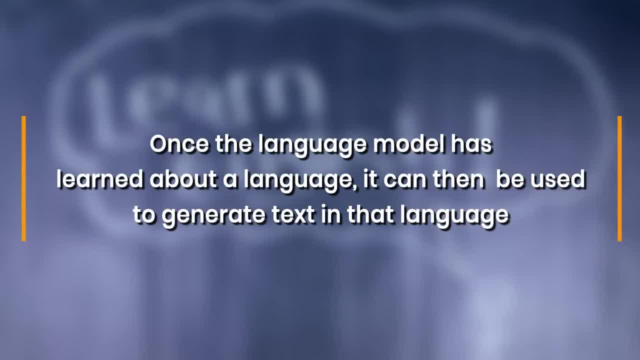 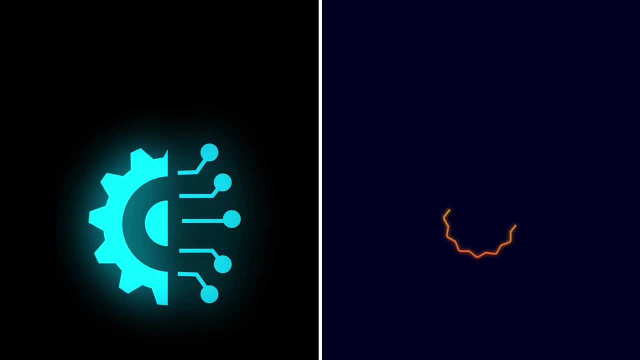 how they are used in different contexts. Once the language model has learned about a language, it can then be used to generate text in that language. Now, Chat GPT provides different language models for different purposes. GPT-3 models, which are: 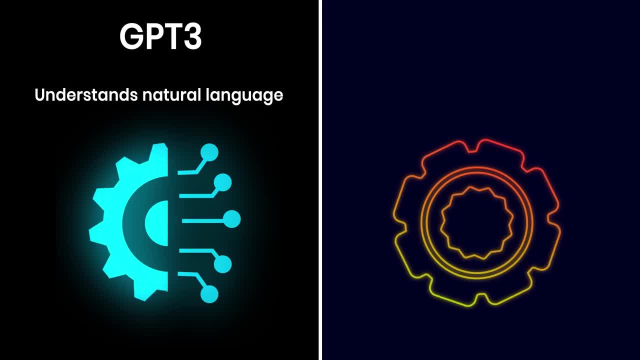 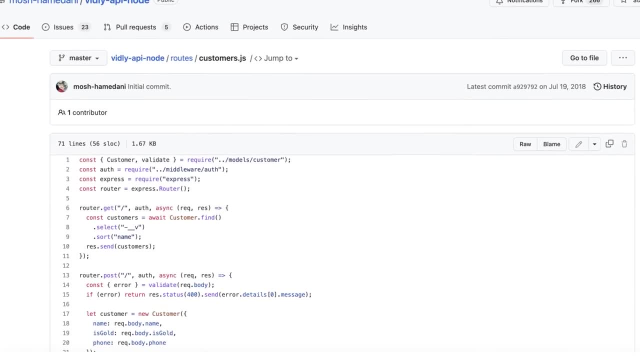 designed to understand and generate natural language like English, and Codecs, which are specifically trained to understand and generate code. These models are trained on billions of lines of code publicly available on GitHub. They're mostly capable in Python, but they're also pretty. 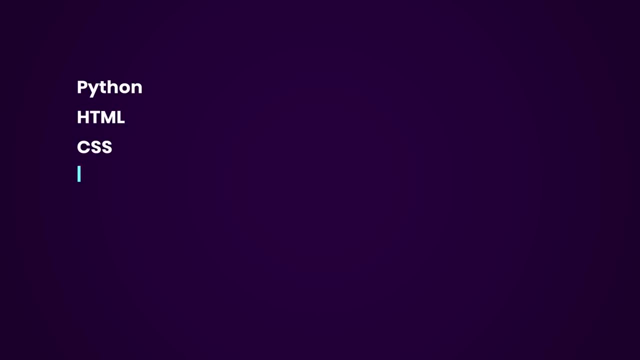 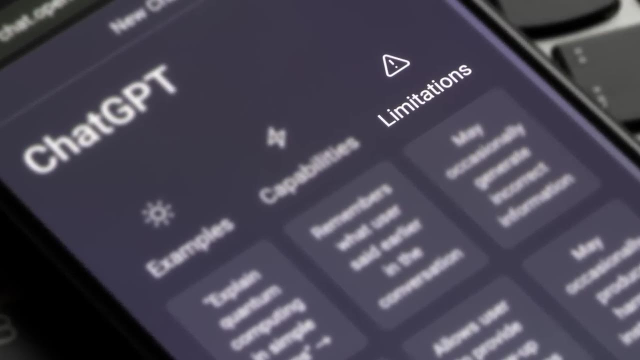 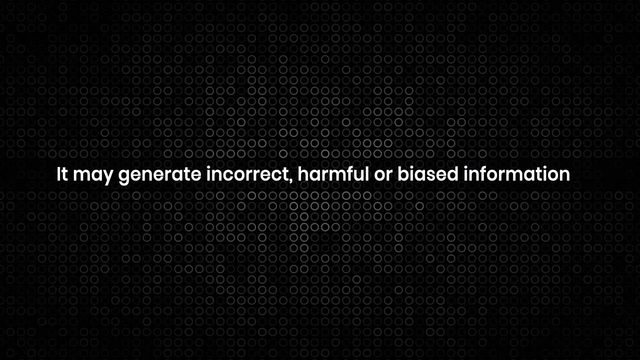 good in a bunch of other languages like HTML, CSS, JavaScript, TypeScript, Ruby, SQL and more. Now, before we look at specific examples, remember Chat GPT, like any tool, has limitations. It might sometimes generate incorrect, harmful or biased information, So don't take whatever it tells you. 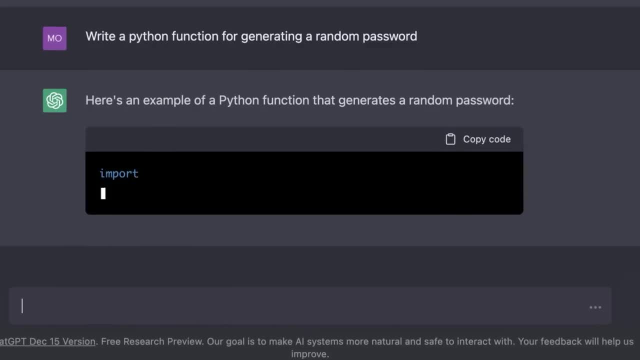 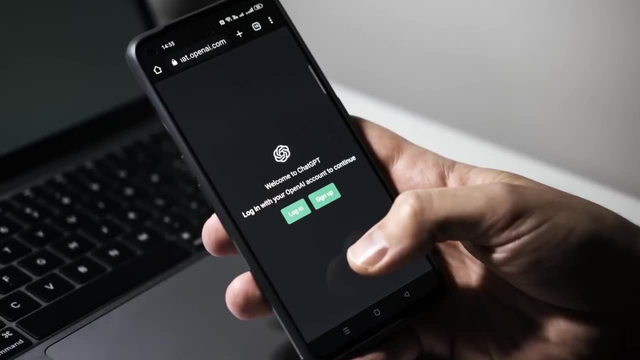 as a silver bullet. Don't use it to learn to code, because the code that is generated is not guaranteed to be right. It might be functional, but it might not be the best way to code. So, in a nutshell, Chat GPT is a powerful tool that can help you be more creative and efficient, but it's not a 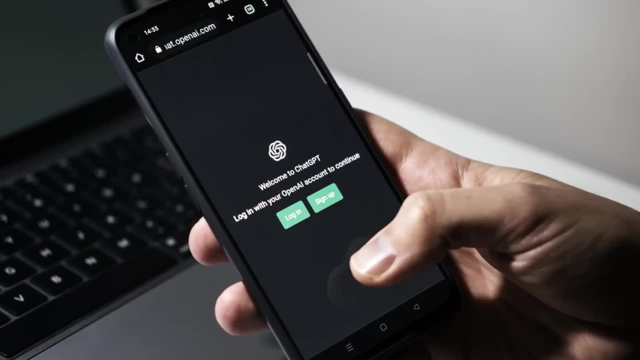 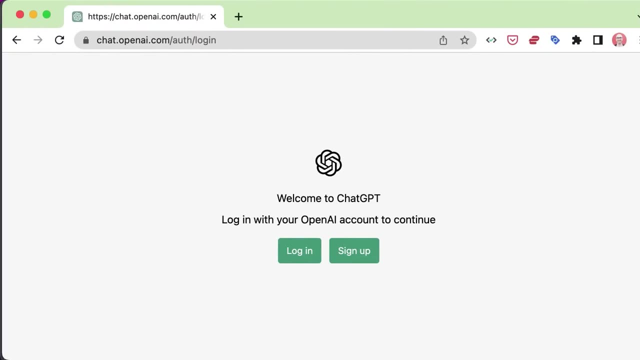 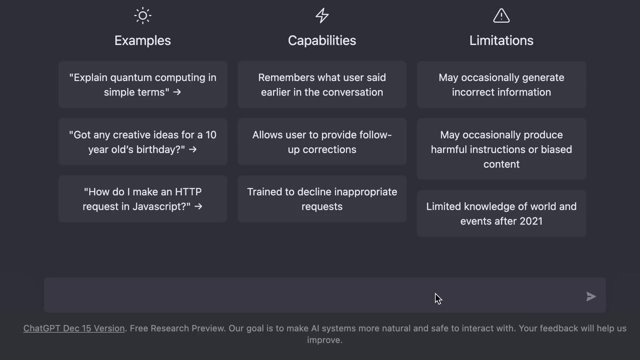 substitute for human expertise and judgment. So that's the theory part. now let's move on and see Chat GPT in action. So head over to chatopenaicom. If you don't have an account, sign up. it takes only a minute. Once you have logged in, you're going to see the main screen with an input box to talk to Chat GPT. 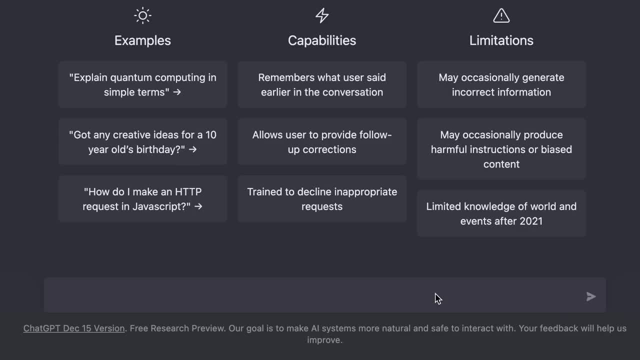 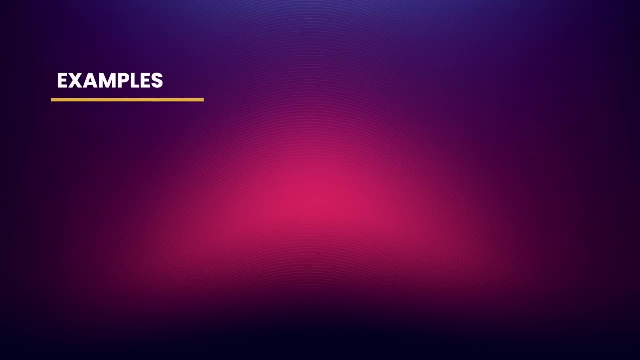 There is also a Chrome extension and a desktop application available. if you don't want to use the web interface, I've put the links down below this video. Alright, now let's get to the fun part. Going forward, I'll be showing you various use cases for different programming. 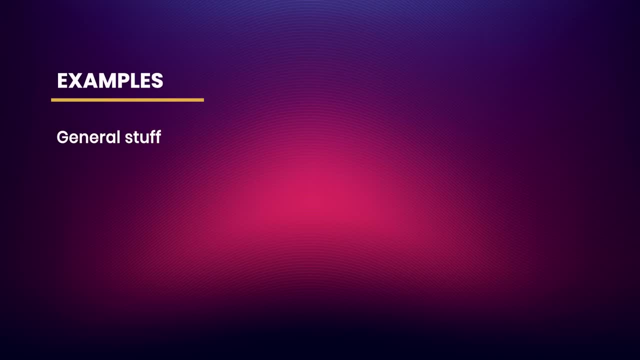 languages. We'll start off with some general purpose questions that apply to anyone, regardless of the programming languages and tools they use. You will see how you can use Chat, GPT to learn new things, write shell scripts, get commands, start a business, write legal documents and so on. Once we cover the basics, then we'll dive into specific examples for front-end, back-end and database development. I will show you examples using HTML, CSS, JavaScript, TypeScript, Python, C++, etc. 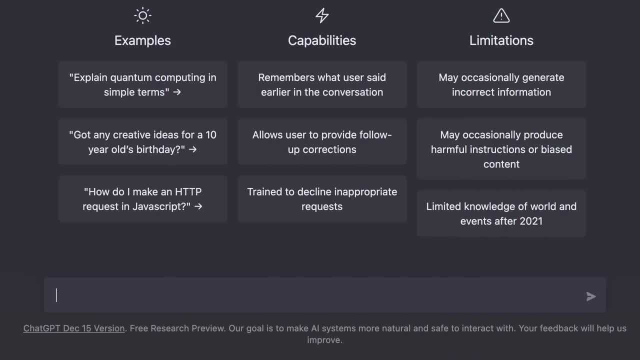 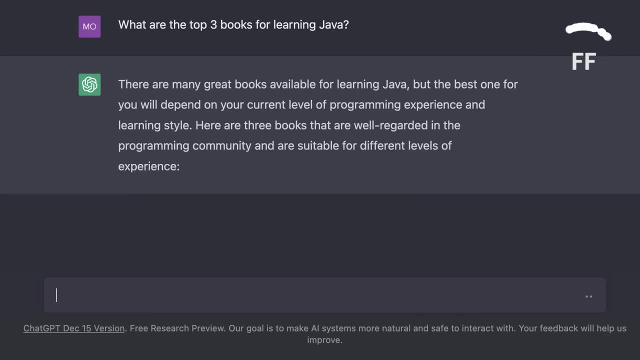 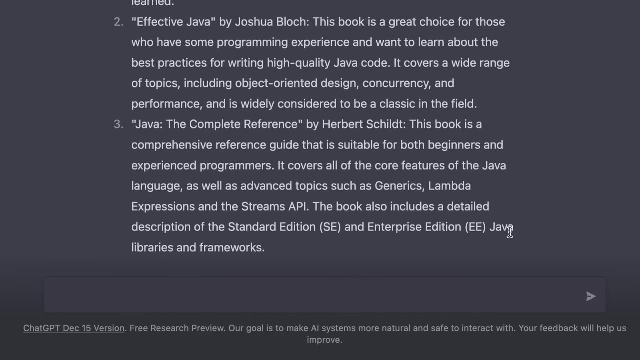 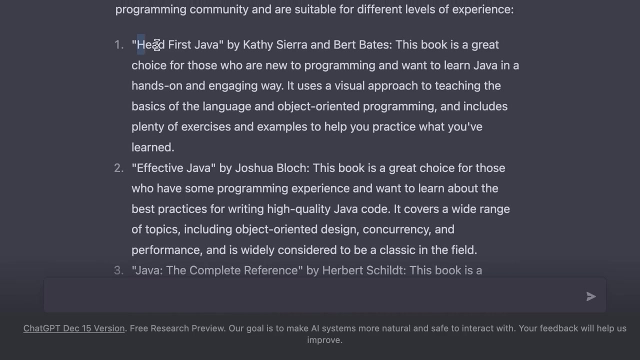 Now here's my first question: What are the top three books for learning Java? Alright, as you can see, Chat GPT has given us a very comprehensive and detailed answer. Now here we can ask more detailed questions. For example, we can ask questions about the first book. 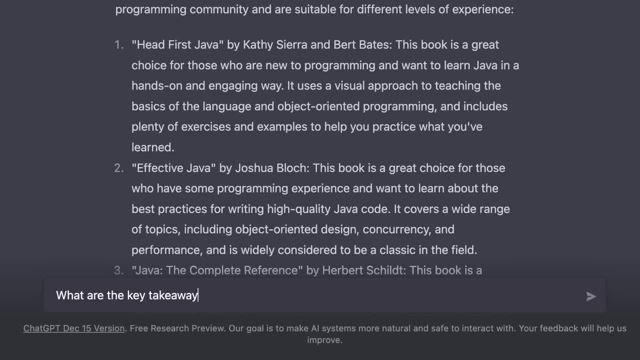 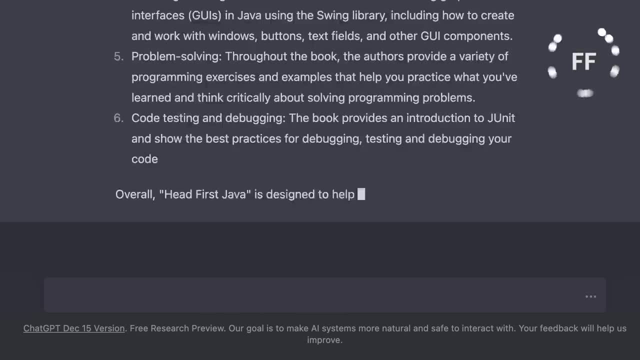 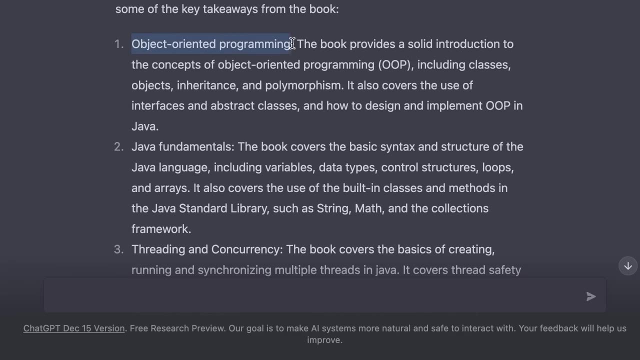 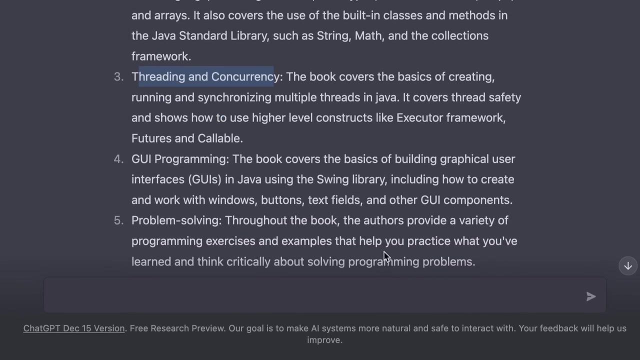 So we can ask: what are the key takeaways for learning Java From head? first Java Alright, another comprehensive answer. you can see that this book teaches you about object-oriented programming, Java fundamentals, threading and concurrency, GUI programming and so on. Now we can also ask: 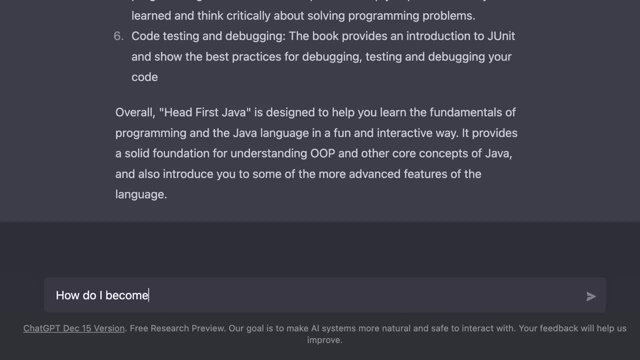 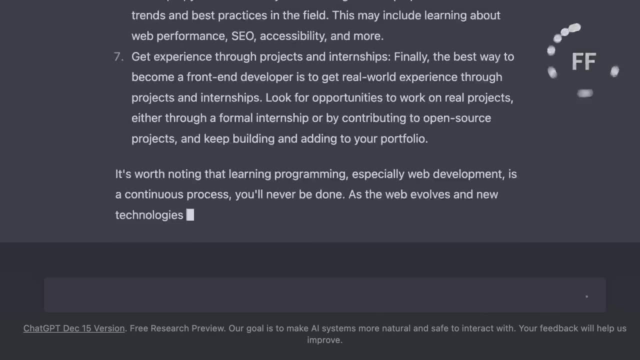 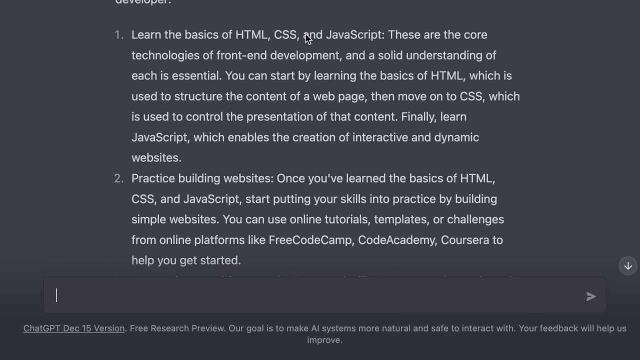 more general questions like: how do I become a front-end developer? So now chat-gpt is saying that to become a front-end developer you need to know the basics of HTML, CSS and Javascript. You should practice building websites, then you can learn a front-end. 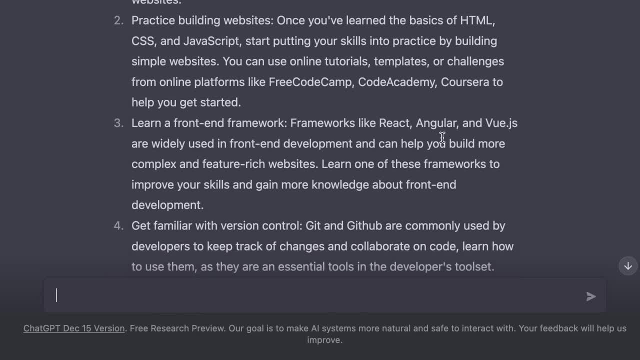 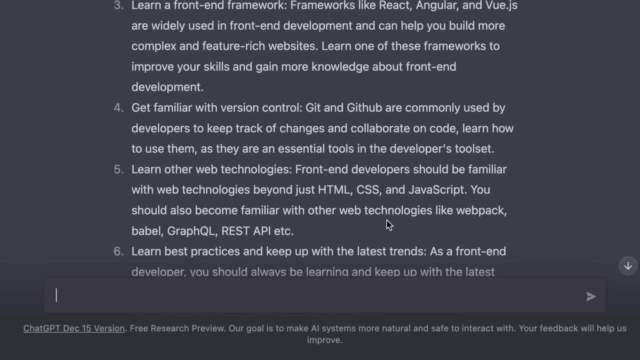 framework like react, angular, Vue and so on. You should also know about version control systems like GitHub and so on. This is almost the same answer you will find on every website that gives you a road map to become a front-end developer. Now let's look at the most popular gifts from Giver, because they give you the way to be a front-end developer. 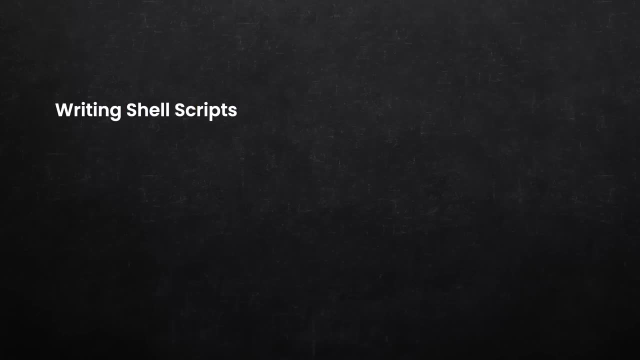 and there's a lot of fun questions on this website and a lot of up and down chat that give you the way to become a front-end developer. Now let's look at more specific examples. We can ask chatgpt to write a shell command for us, For example. we can say: write a bash command. 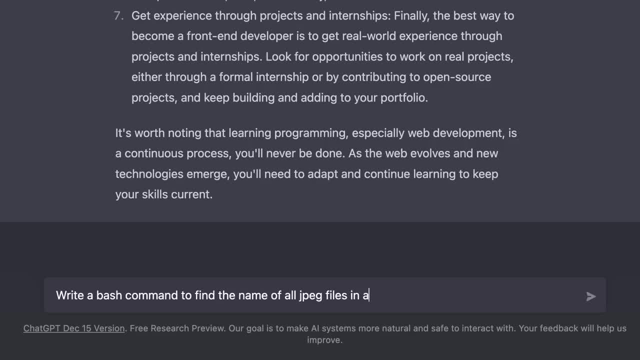 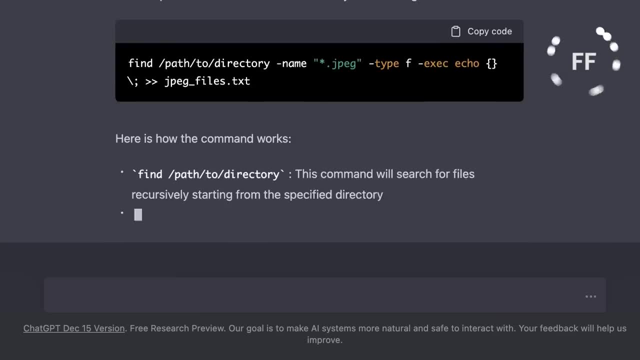 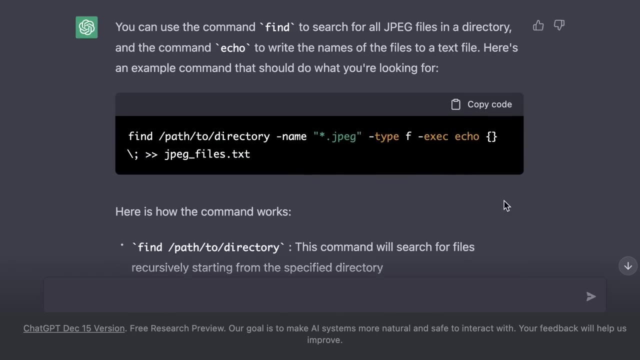 to find the name of all jpeg files in a directory and write them all to a text file. Take a look, I love this answer. So if you're not good with Linux commands, you can easily find the final instruction you should use to solve that problem. but what is beautiful. 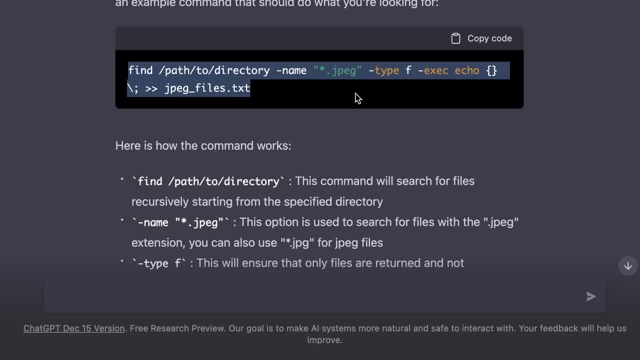 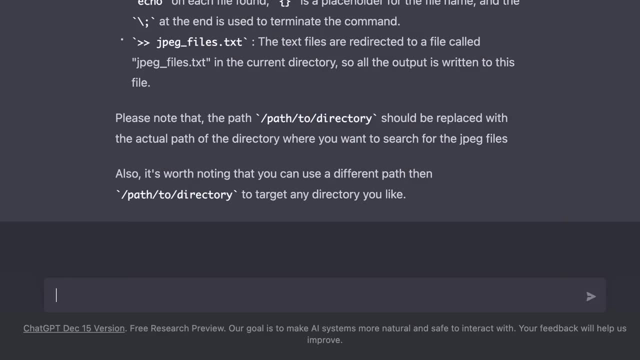 about chatgpt is that it also explains how this command works, line by line, piece by piece. We can also have chatgpt write git commands for us. For example, we can ask: how do I know how many lines of code I've committed? 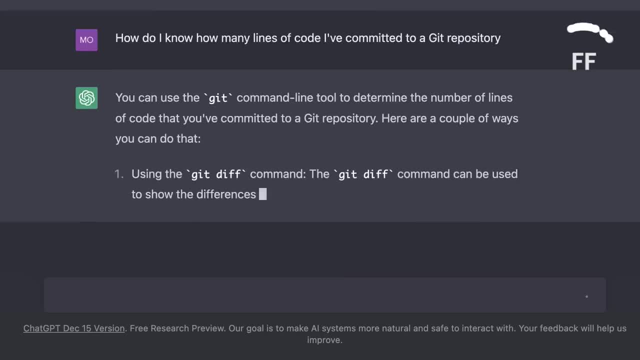 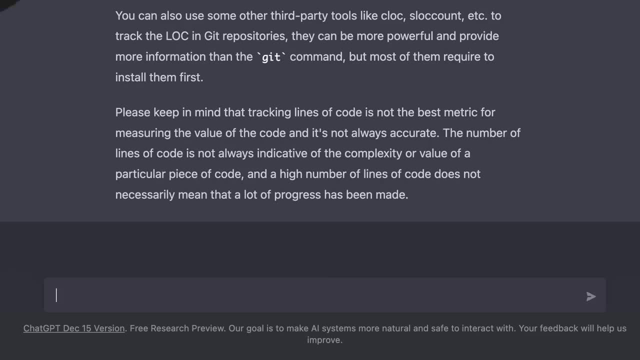 to a git repository. We can also use chatgpt to create creative. For example, let's say you want to start a business, You can have chatgpt generate app or website names for you. For example, we can say: I want to make a revolutionary online. 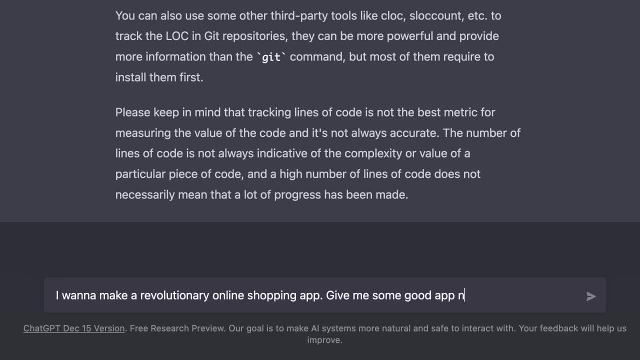 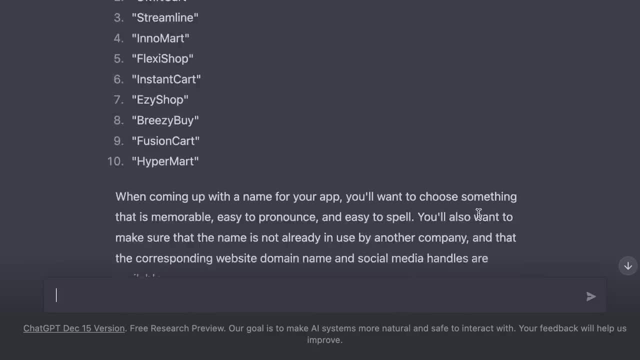 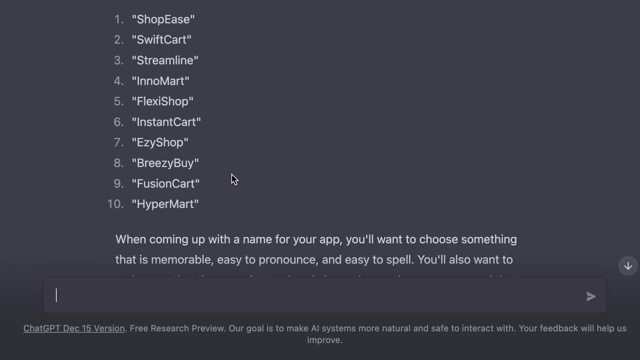 shopping app. Give me some good app names. So chatgpt is suggesting names like shop is swift, cart, streamline and so on. I think this list is pretty damn good. These are just some example prompts. you don't need to use the exact same wording to talk to. 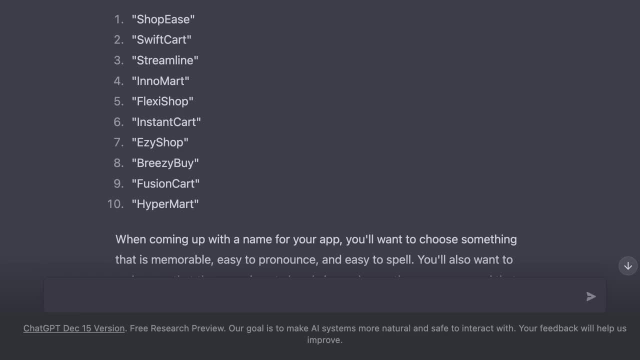 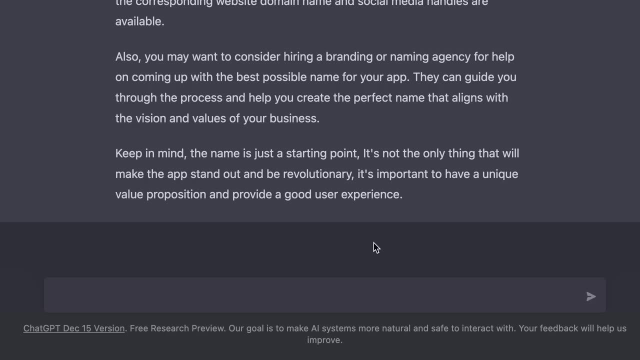 chatgpt. you can ask any questions you want in your own way. Now, if you have used this tool before, let us know in the comments below the interesting questions you have asked, so we can all learn and inspire each other. We can also ask chatgpt to write contracts for us. Here's: 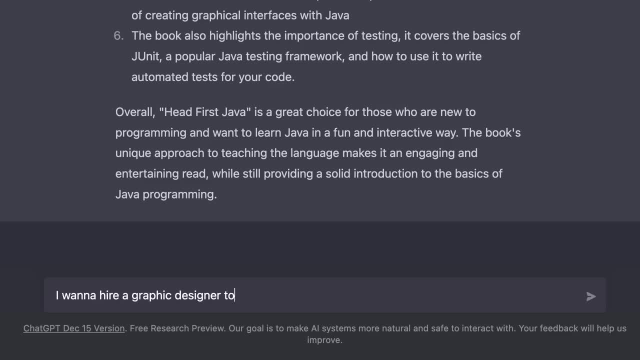 an example: I want to hire a graphic designer to design a website. We have agreed that they will deliver the first draft in two weeks and offer three iterations free of charge. Any iteration after will be charged at $50 an hour. Write a contract. 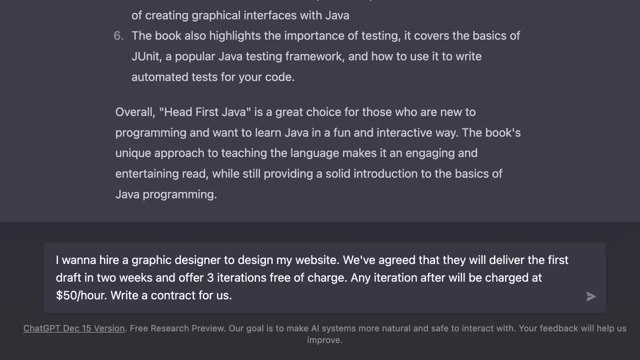 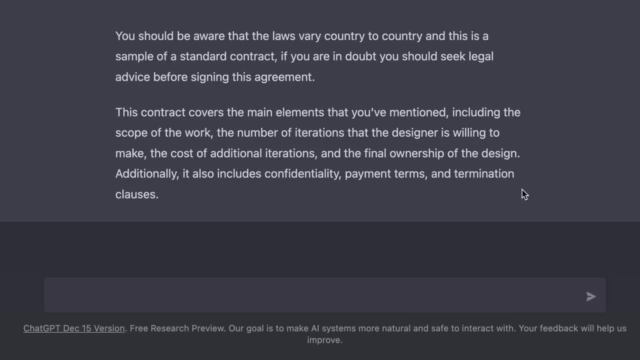 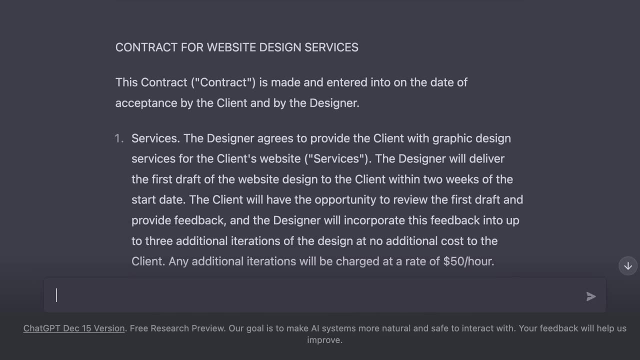 for us. So the more details we give to chatgpt, the better response we'll get. Alright, take a look. This is a pretty damn good contract to start with. Of course, you don't want to take this as is and use it in the real world without first passing it by a real 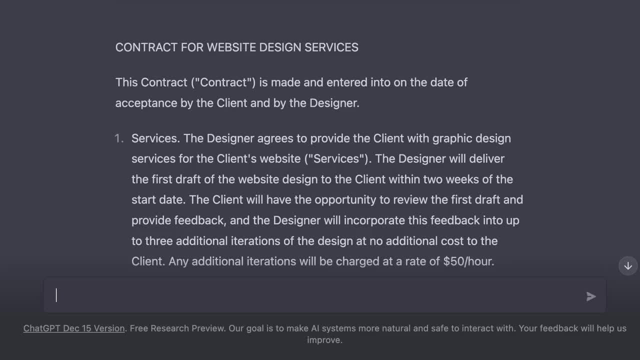 lawyer. that's why, earlier, I told you that ChatGPT is not a replacement for humans, at least not at the moment. It's just a way to increase your productivity and get things done in less time. Now, if you're applying for a job, there are a number of ways ChatGPT can help you. For example, 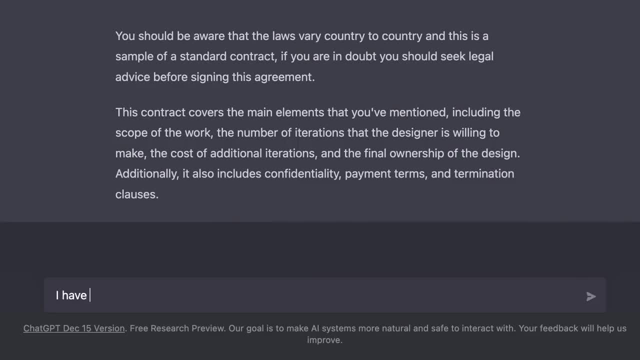 you can have it. write a resume for you. Here we can say: I have three years of experience coding in HTML, CSS and JavaScript. Write a resume for me. Of course we can give it more details. we can explain our education level. 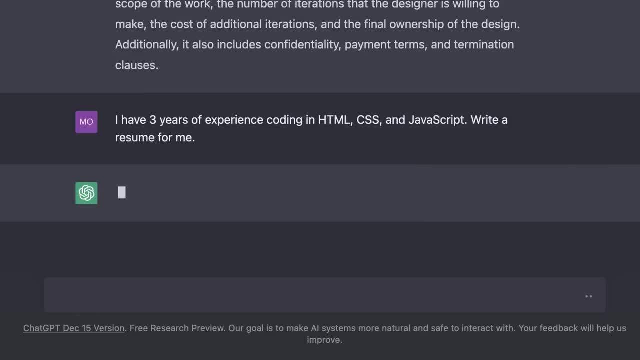 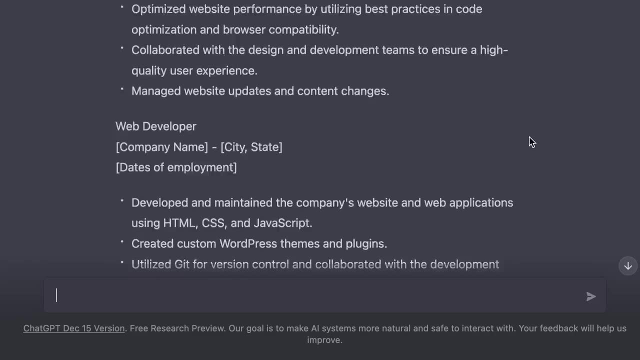 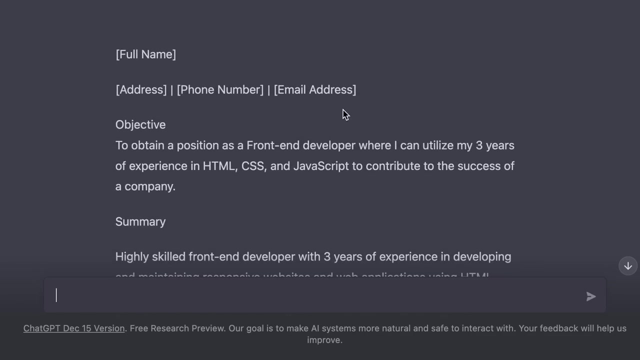 our past projects and so on, But look at what we get with this simple prompt. Alright, take a look. So ChatGPT created a basic layout that includes our name, address, phone number, email, some objective summary technical skills. 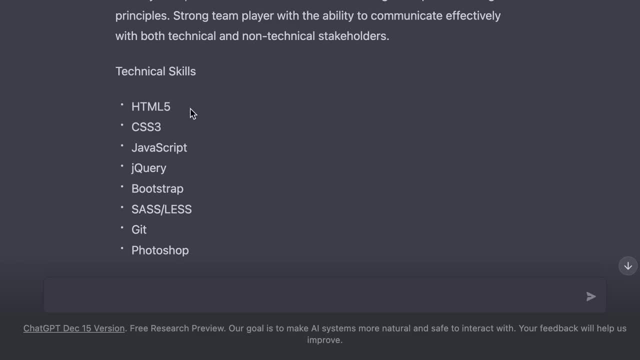 and it has already listed all the related web technologies. So we have HTML, CSS, JavaScript, jQuery, Bootstrap. we didn't mention any of this, but it assumed that we have these skills. It also included a section about professional experience, including past. 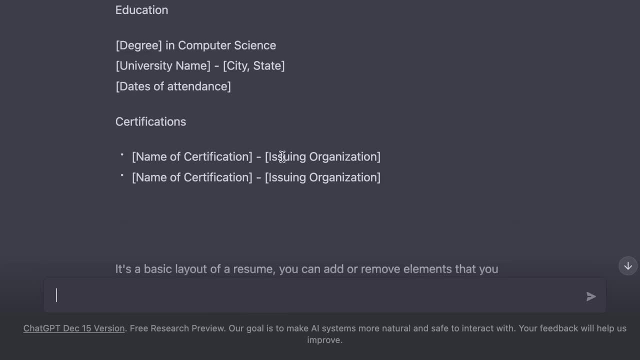 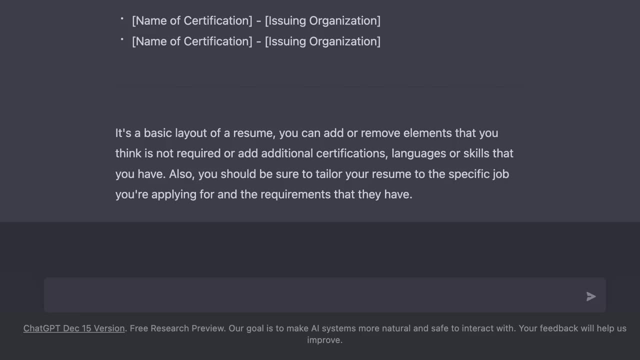 projects, as well as education, certifications and so on. Again, it's a great starting point. Now, let's say you're applying for a front-end developer role. You can ask ChatGPT to write a cover letter for you. 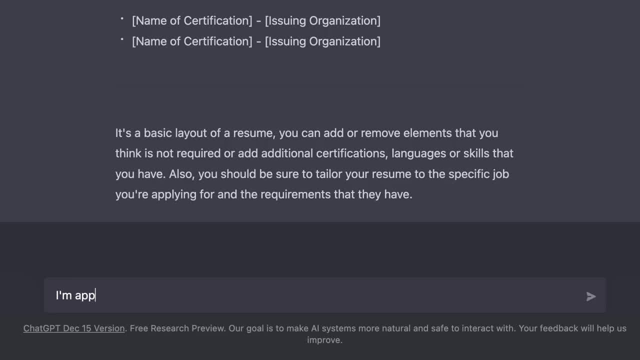 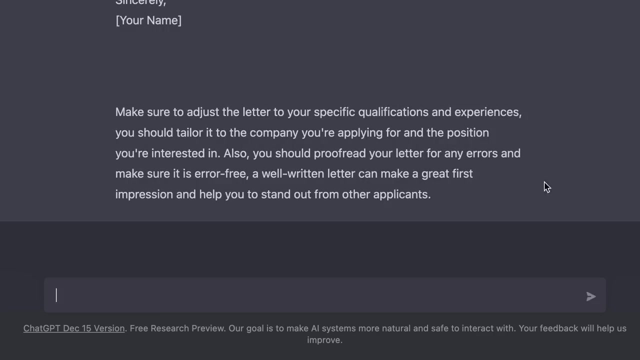 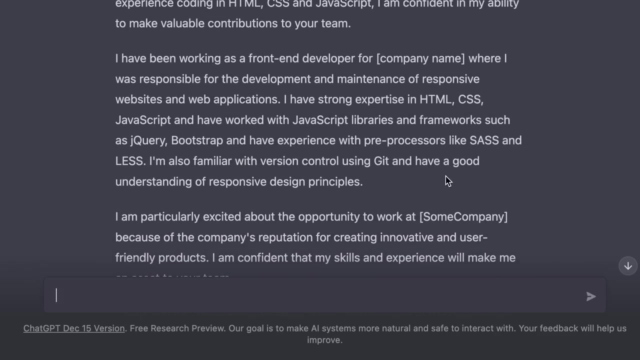 that you can email to that company. So we can say: I'm applying for a front-end engineer role at some company. write a cover letter for me. Alright, take a look, We have a comprehensive cover letter, beautifully written, in perfect English. How good is that? Now let me show you another fun one. 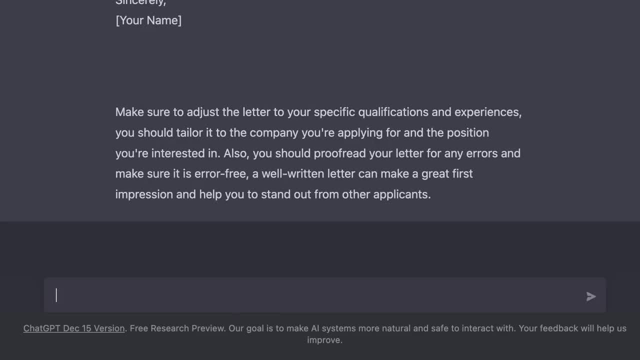 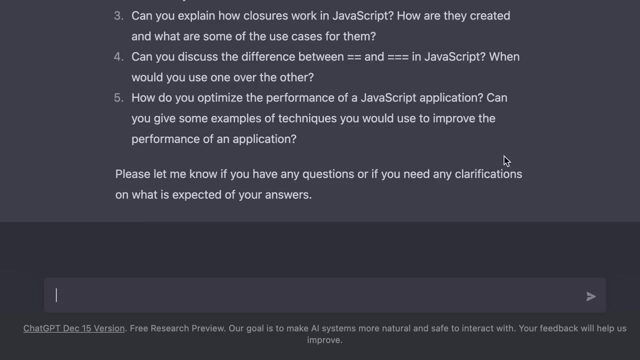 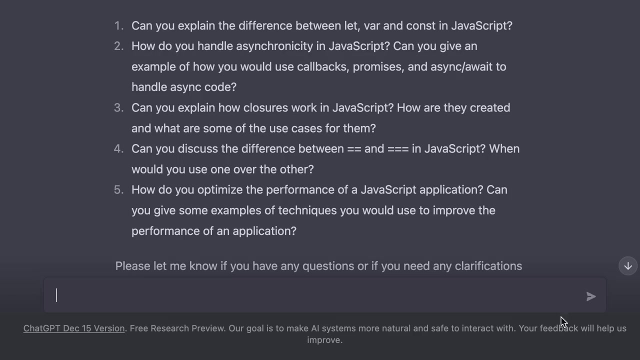 You can have ChatGPT ask you interview questions. We can say, act as a technical interviewer and ask me five questions about JavaScript. Take a look, Alright. so here we have five questions that are often asked in technical interviews. Now, let's say you don't know the answer to the first question You can ask. 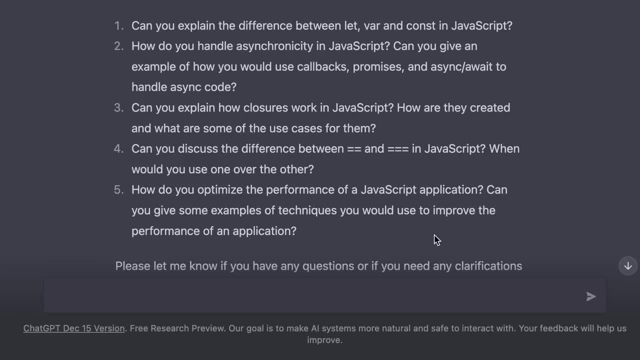 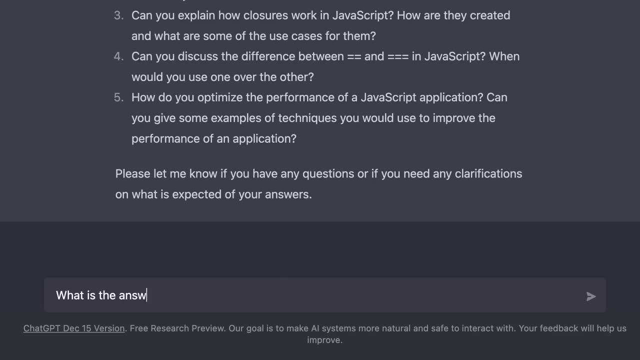 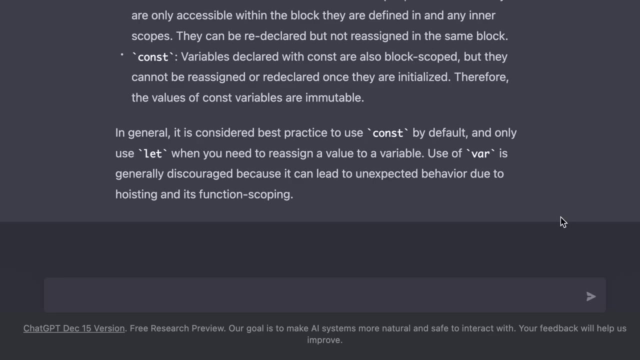 a follow-up question. So the beauty of ChatGPT is that it remembers everything you have told it in this conversation thread. So here we can say what is the answer to the first question. Again, we get a very comprehensive, detailed answer. You can also ask ChatGPT to help you. 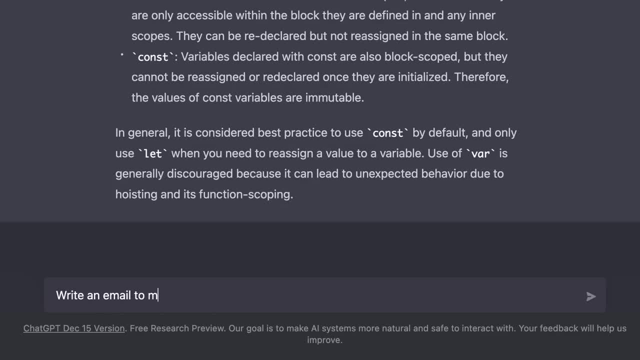 write emails. For example, we can say: write an email to my boss asking for a raise. I've worked at this company for two years and successfully delivered several emails. So here we can say what is the answer to the first question. 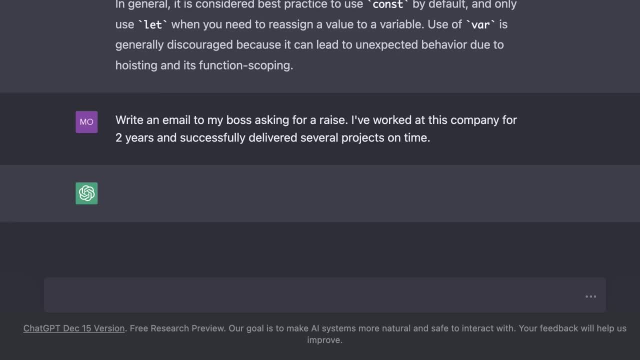 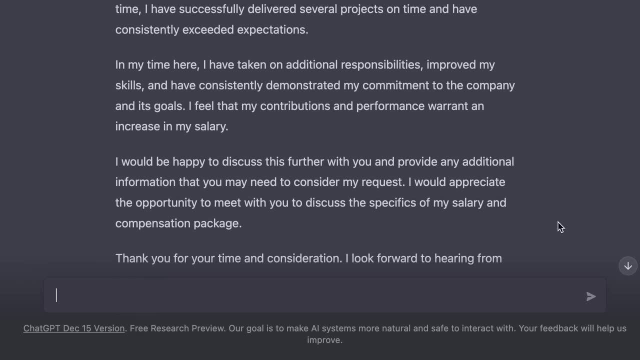 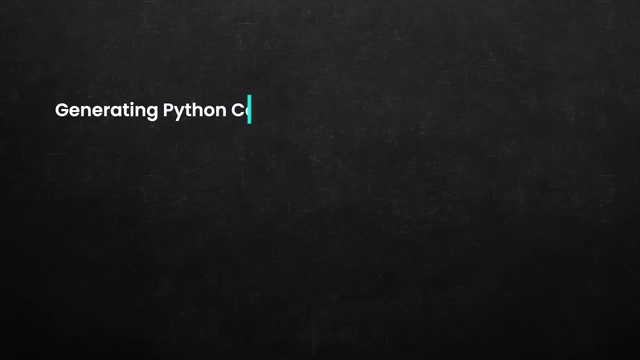 Projects on time. Seriously, if I wanted to write this myself, it would take me 10 to 15 minutes, if not longer. I got the answer in just two seconds. Alright, now let's look at a few examples involving code. 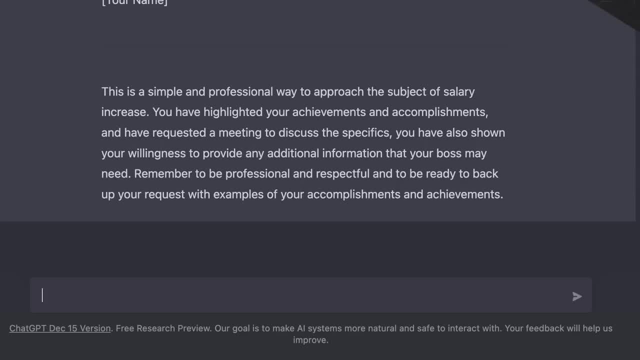 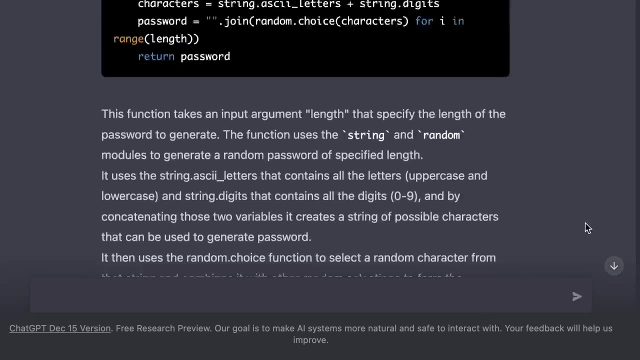 We'll start with using Python for writing a command line tool. We can say, write a Python function for generating a random Python. So, as you can see, we get a piece of code beautifully highlighted with an explanation of how it works. Now, if there's a part of this code, 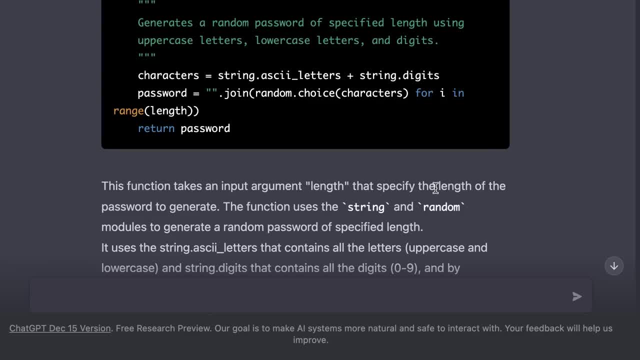 that you don't understand. you can always ask follow up questions. For example, we can ask what this expression does in this code. So we can ask: what does 4 in i range of length do in this code? So we can ask: what does 4 in i range of length do in this code. 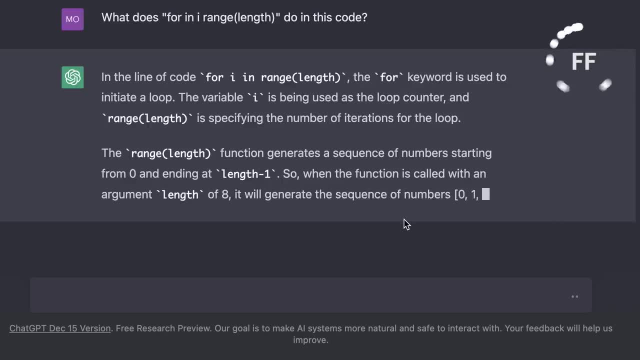 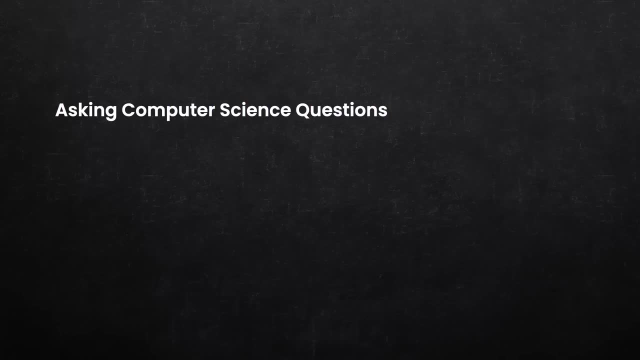 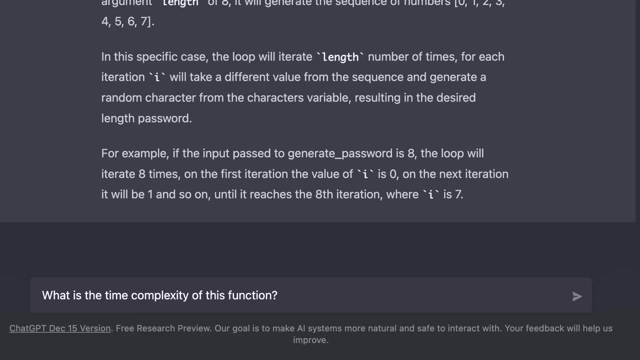 Take a look, Really, really useful. Couldn't be better. Now we can also ask computer science questions like: what is the time complexity of this function? Now, if you're not familiar with this concept, time complexity is a way to explain how. 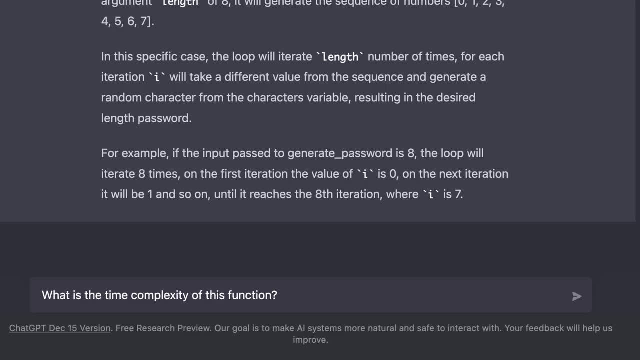 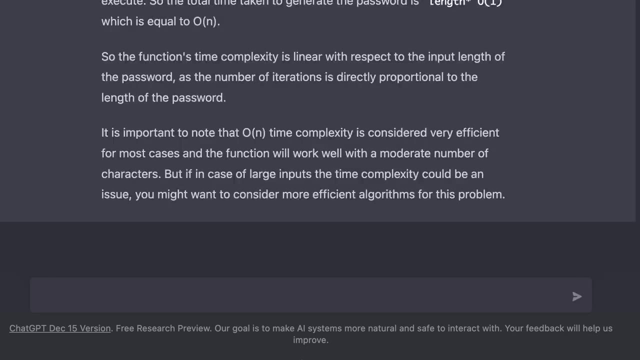 large inputs impact the performance of an algorithm. It's really beyond the scope of this tutorial. I've covered it in detail in my data infrastructure course, in case you're interested. So let's see what we get. So chatgpt is saying that this function's time complexity. 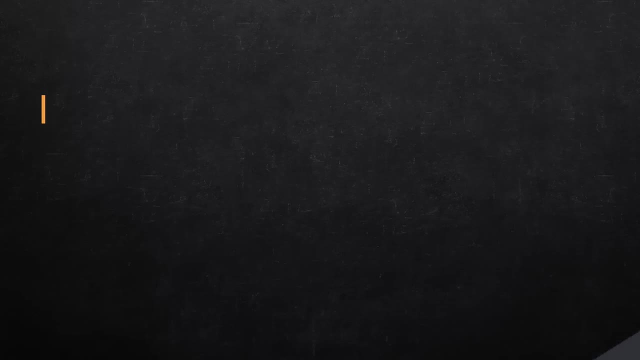 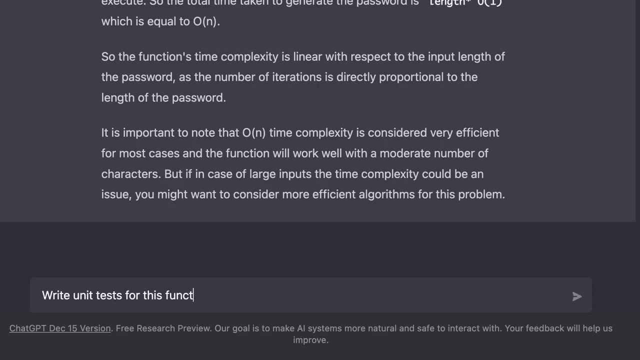 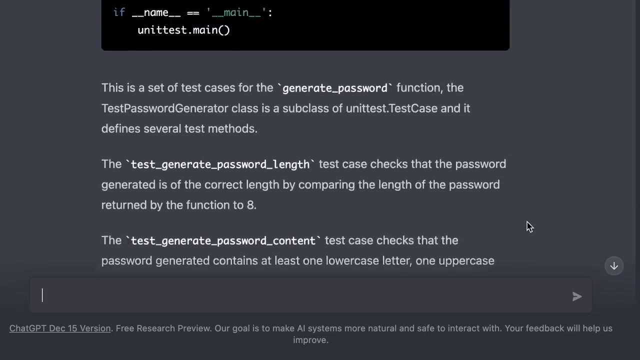 is linear. Now let's take this to the next level. We can ask chatgpt to write unit tests for this function. So write unit tests for this function. Seriously, how good is this? Seriously, how good is this? 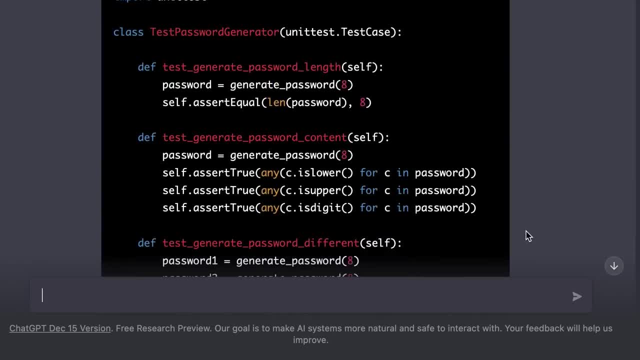 Seriously, how good is this this? if I wanted to write all these unit tests by hand, it would take me probably 20 to 30 minutes, if not longer. Of course, we should always use our own judgment to make sure that the tests are correct, but I think this code is a great. 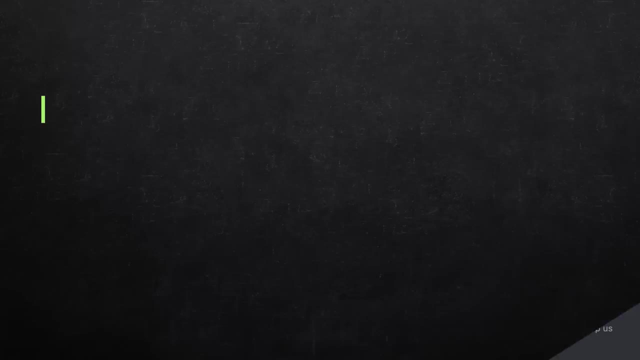 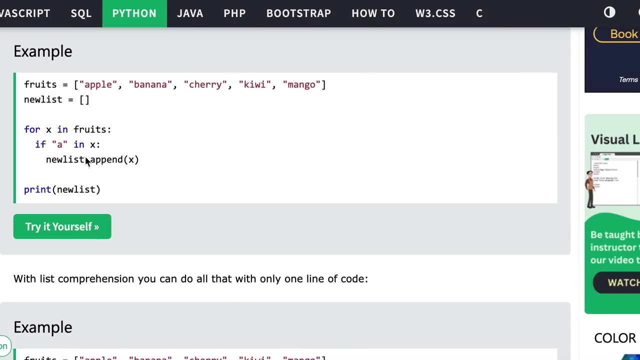 starting point and it really saves us a lot of time. We can also ask chat GPT for ideas to improve our code. For example, here on w3schoolscom we have this piece of python code where we use a for loop to iterate over a list of. 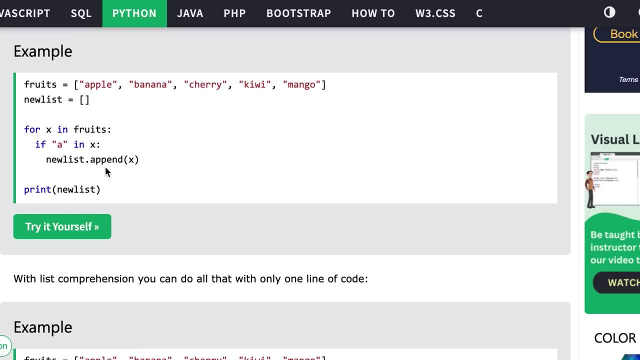 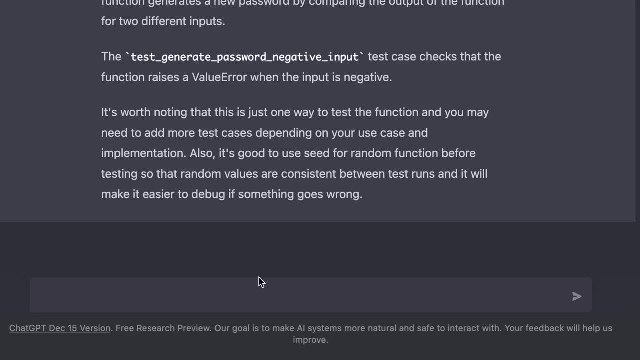 fruits. if the fruit has a in it, then we add it to a new list. I'm going to copy this code and give it to chat GPT to see how we can improve this code. So take a look, How can I improve this code? Now, here we should hold. 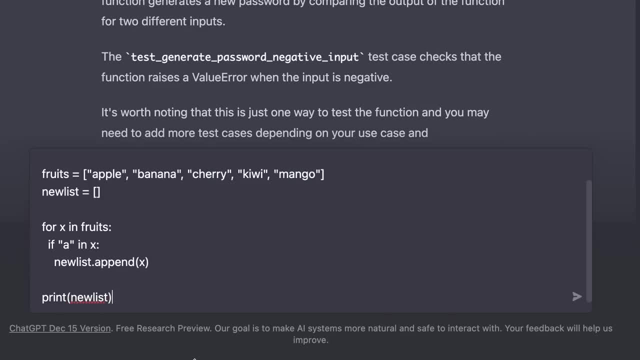 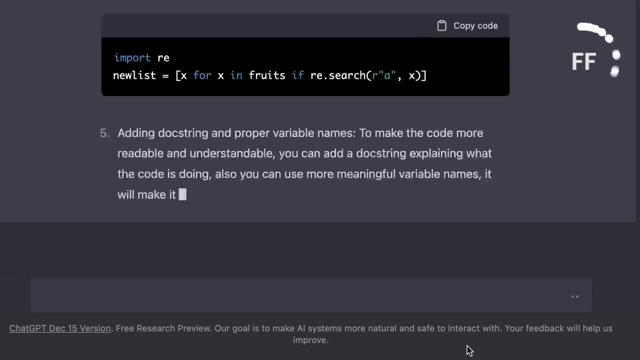 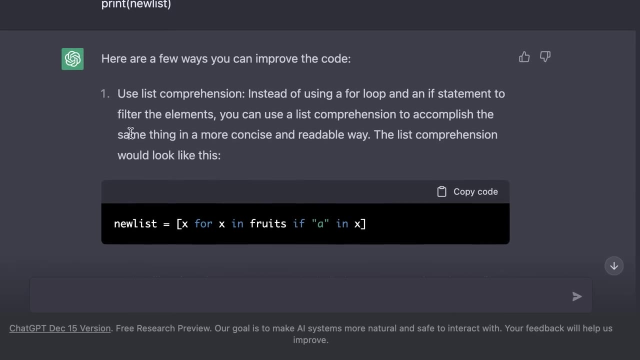 shift and then press enter. so we go to the next line. now we paste our code and then press enter to submit the question. Alright, look a lot of details, absolutely amazing. One thing I love here is that chat GPT is suggesting to use a list comprehension, which is a one. 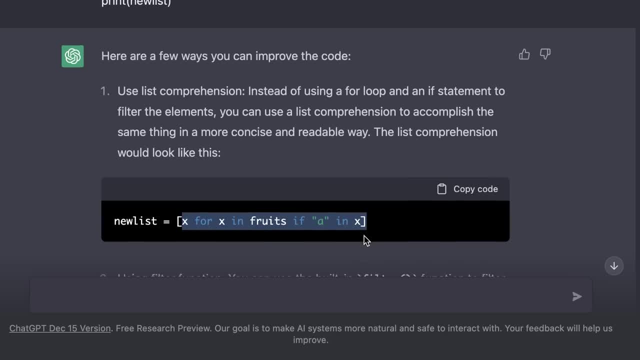 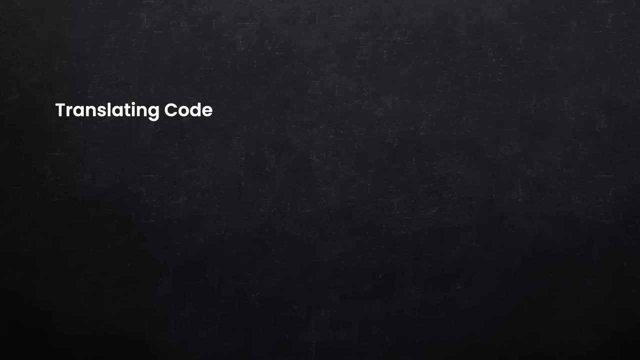 liner for implementing the same logic. Of course there are more ways to improve this code. we're not going to get into details here. We can also ask chat GPT to convert our code from one language to another. For example, we can say: convert this python code to javascript. 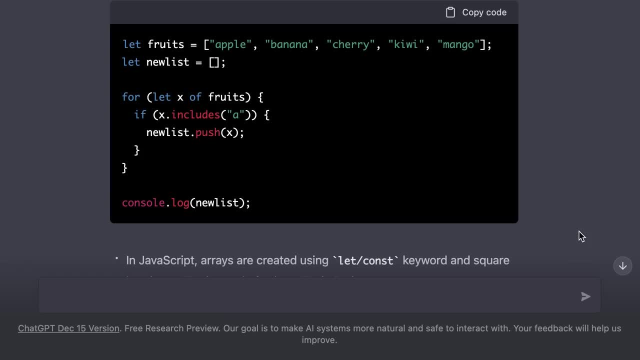 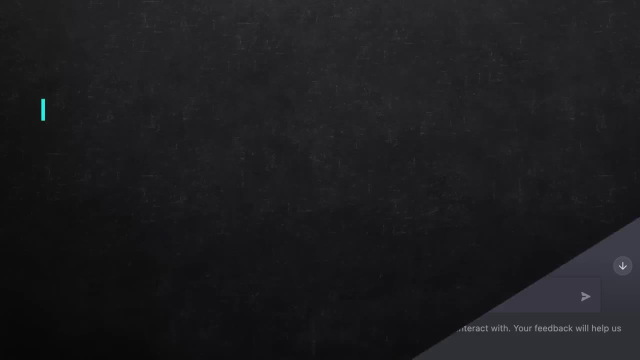 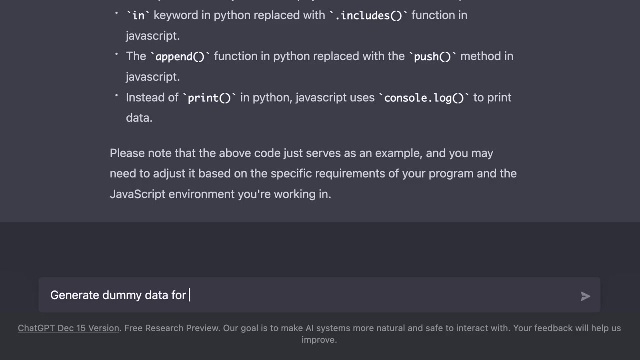 Incredible. in just a few seconds our code was converted to javascript and down below we have all the details about how this code works. We can also use chat GPT to generate dummy data. For example, we can say: generate dummy data for a table called customers. 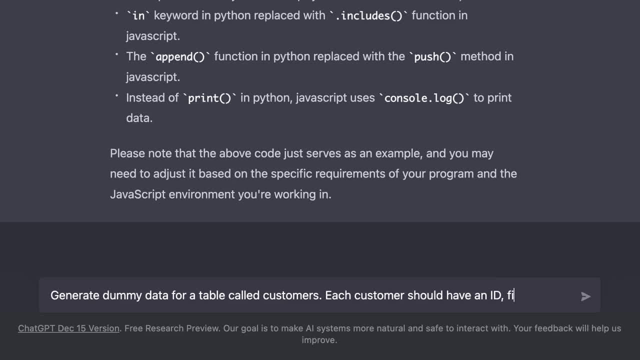 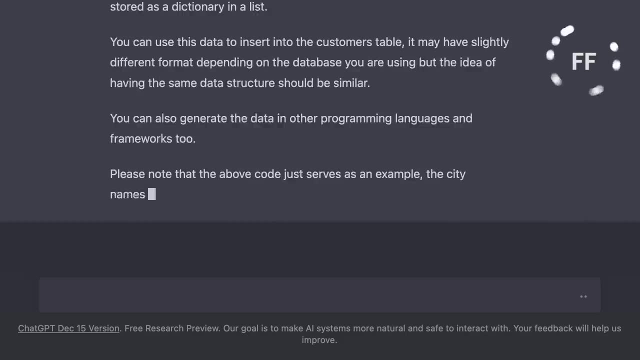 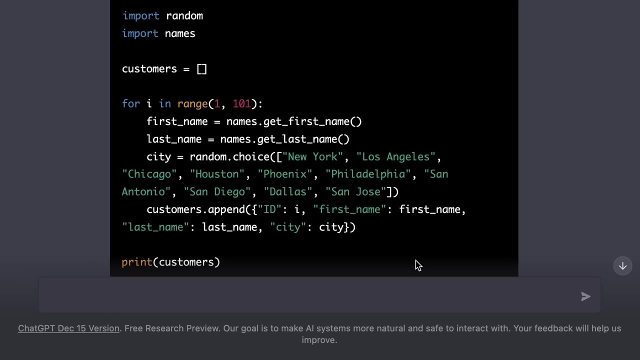 each customer should have an id, first name, last name and city. Now, in this case, chat GPT gave us a python script for generating dummy data. but what if we want the actual data, not a python script? We can say: 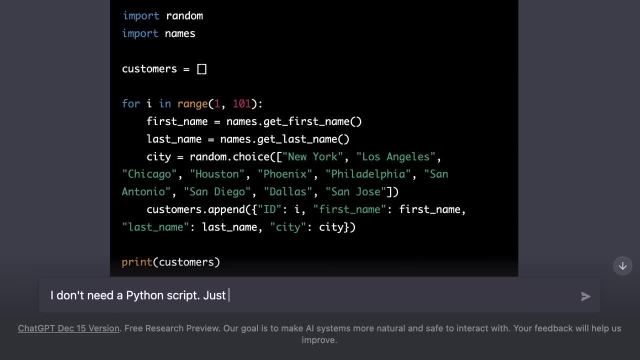 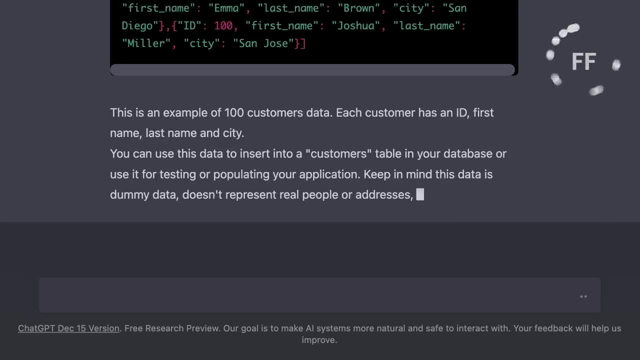 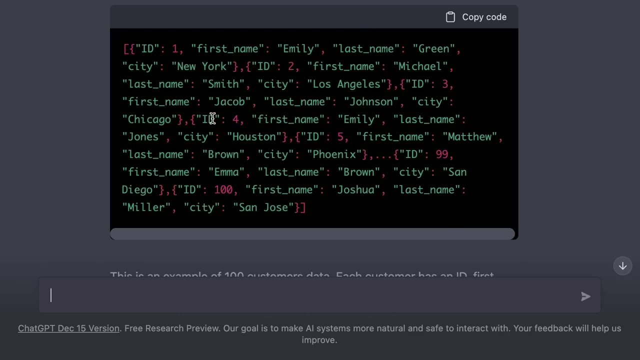 I don't need a python script, just give me the data. So now we get a list of 10 people represented using the JSON format. Now we can take this to the next level and say: create a python class for storing these objects. 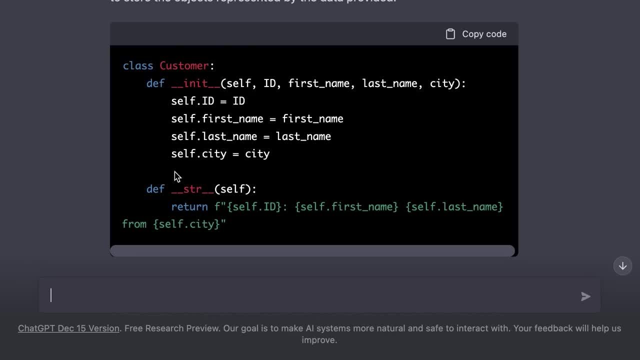 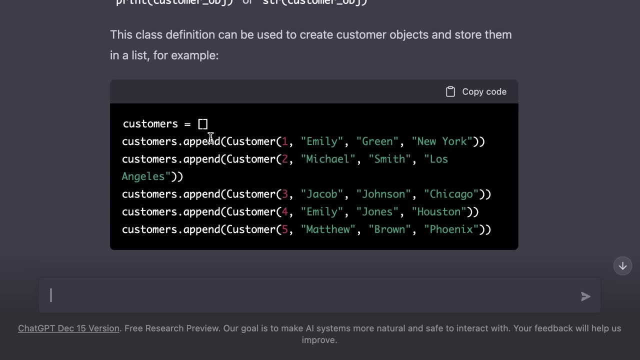 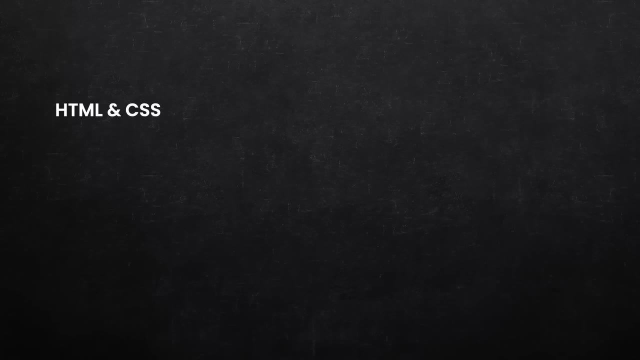 Alright, look, we get an example of a python class called customer, along with how we can use this class to store a bunch of customer objects inside the list. Absolutely beautiful. Now, if you're a front-end developer, you can ask chat GPT to generate some HTML markup for you. 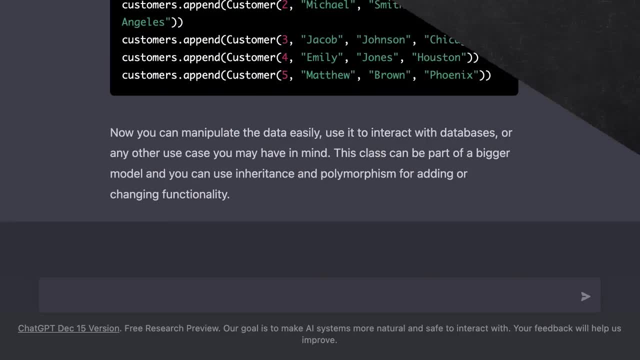 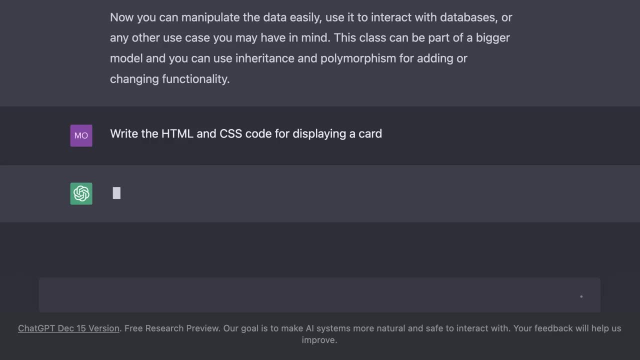 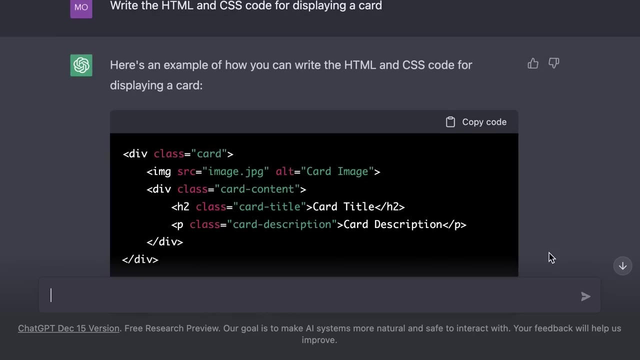 And this is where examples get more and more interesting. For example, we can say: write the HTML and CSS code for displaying a cart. Alright, take a look, we have the markup here. we have a div with a class of cart. inside the div we have an image. then we have the cart. 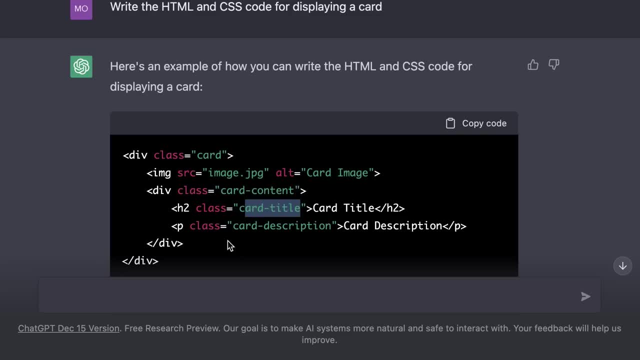 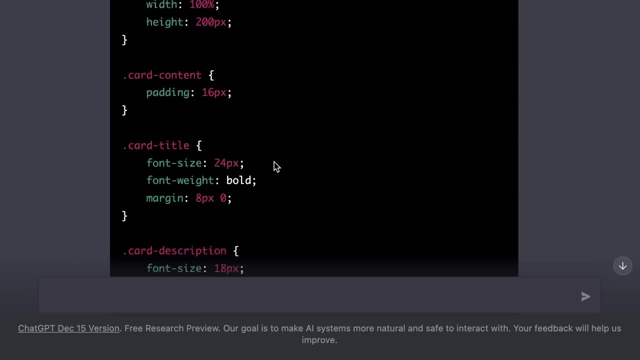 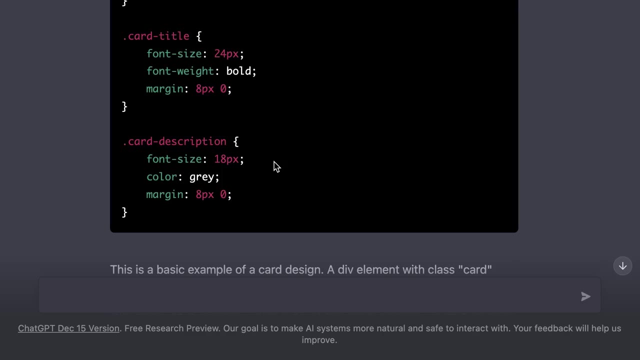 content. inside this div we have the cart title and cart description. This is really good, And right below that we have all the CSS we need to display a beautiful cart. Of course, we probably need to customize this, but again, this is a great starting point. Now we can stop here. 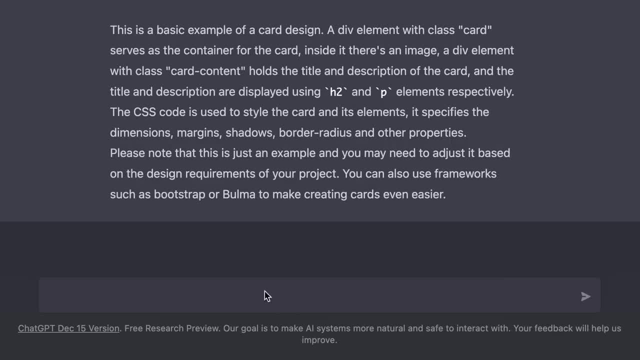 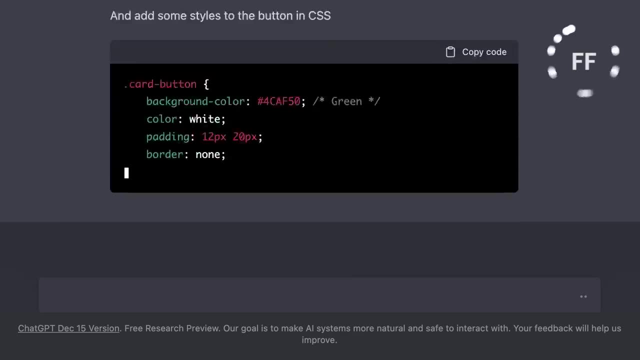 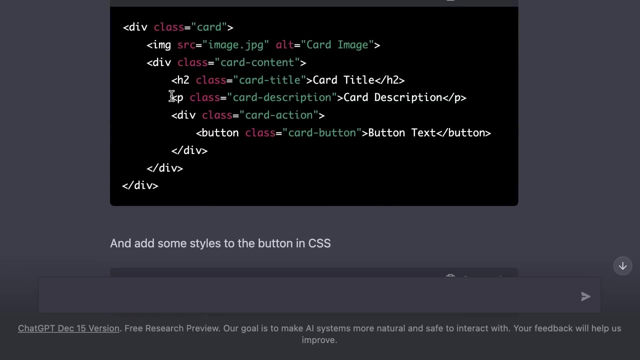 or we can customize this further. For example, we can say: add a button below the cart content. Alright, look what happened. So now we have a new markup right on top of the cart content. Under the cart description we have a new div with a class of. 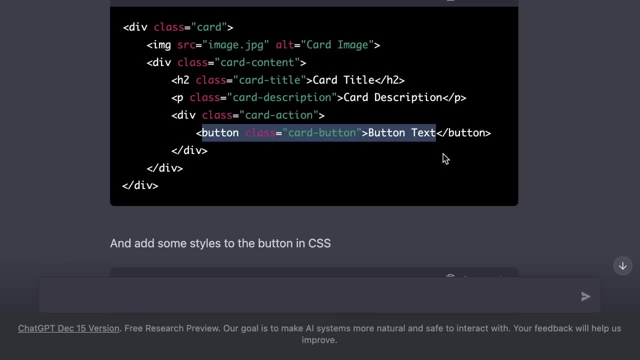 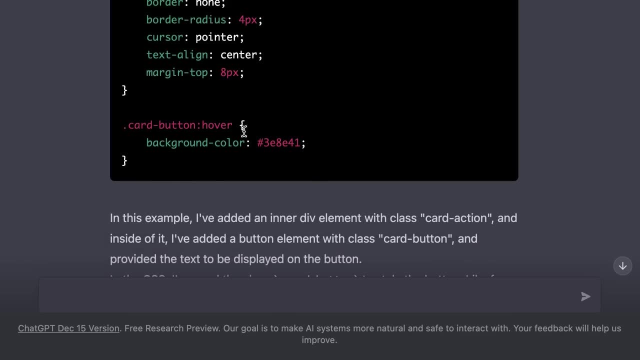 cart action, and inside this div we have a button- beautiful. Now we also have more styles for this button. we have the plain styles as well as the styles for the hover effect. Now let's take this to the next level. We can say: when I hover, 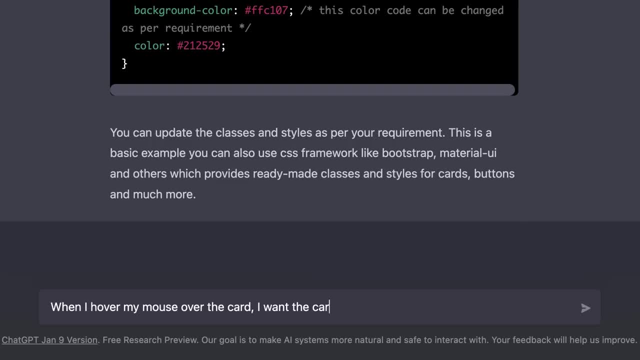 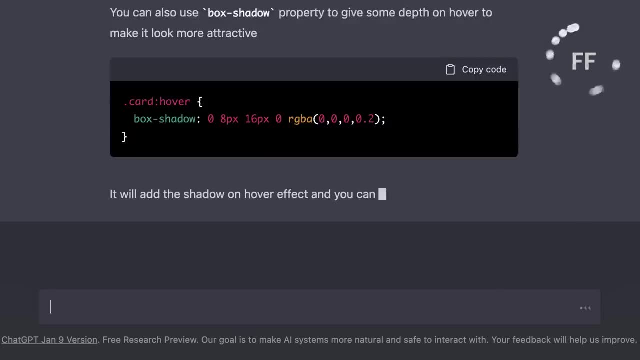 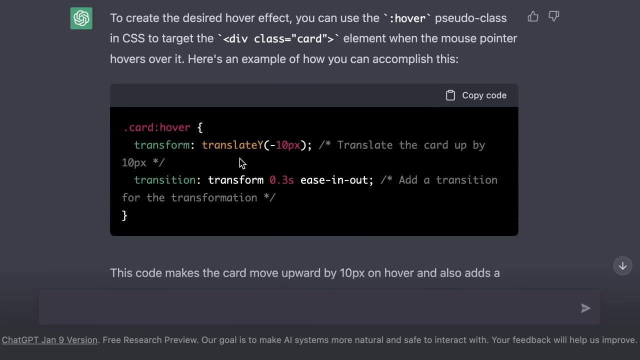 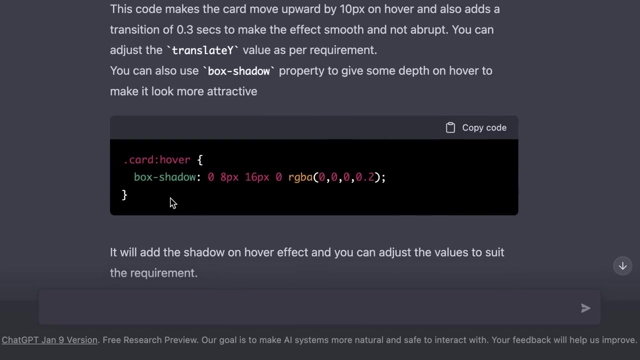 my mouse over the cart, I want the cart to slightly slide up. So chat GPT is suggesting that we should use the hover pseudo class and the translate function, translate y- to slide the cart up. Beautiful, I love it. It's also suggesting an alternative solution using box shadow, so it's pretty. 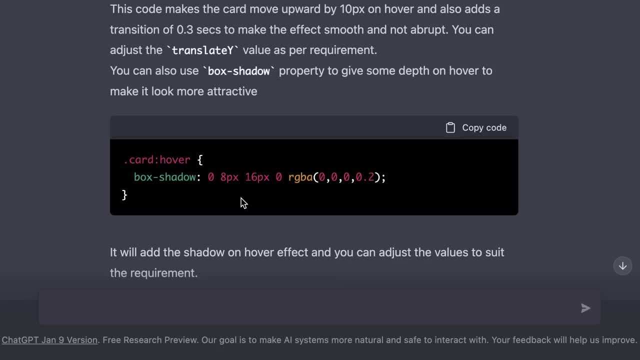 up to speed with CSS features. Now let me show you something really cool. We can ask chat GPT to rewrite this code using Tailwind CSS. If you're not familiar with Tailwind, it's a CSS library that has gained a lot of popularity lately. So here we can say: 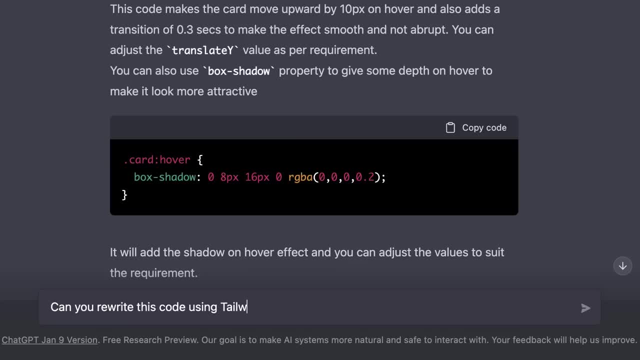 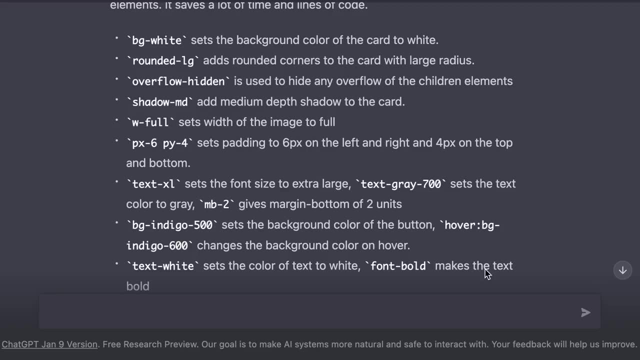 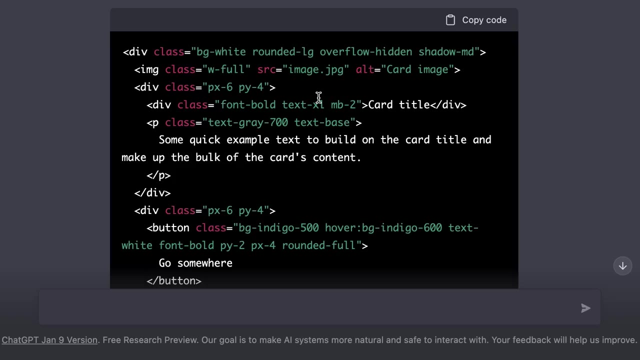 can you rewrite this code using Tailwind CSS? There you go. Now we have the same markup, but with the utility classes that come with Tailwind CSS, So we don't have to create CSS classes anymore. Now, here we can get more creative and see what. 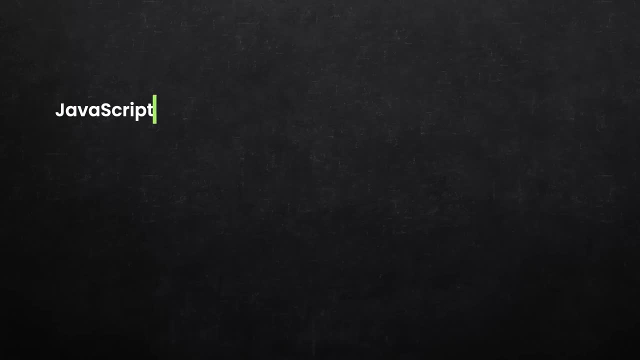 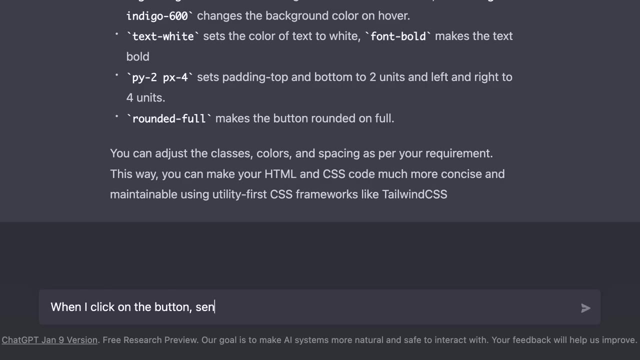 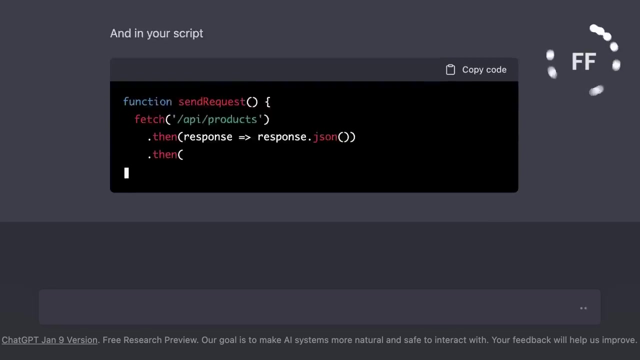 other UI libraries are supported. Next, we can bring some JavaScript to the mix and make this interactive. So we can say, when I click on the button, send an HTTP request to slash API, slash products. Alright, let's look at the generated code. So chat GPT. 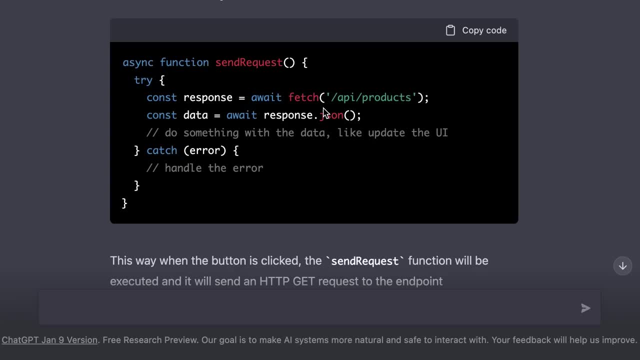 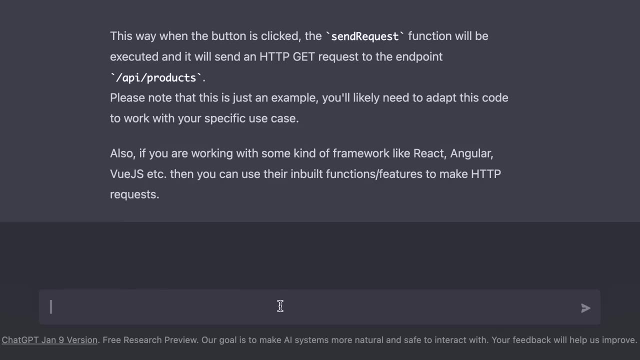 is suggesting to use the fetch API. that is supported in pretty much most modern browsers, but I personally don't like to use the fetch API. So I'm going to customize this further and say: instead of the fetch API, use Axios, which is a library. 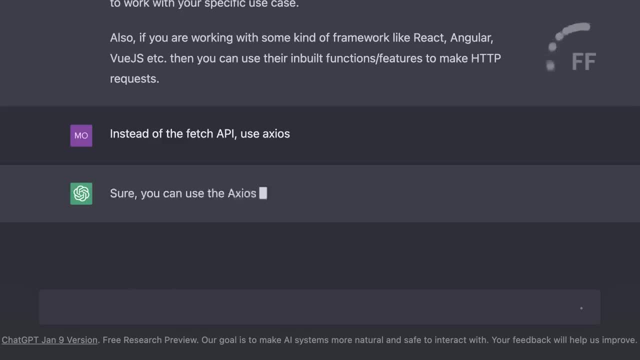 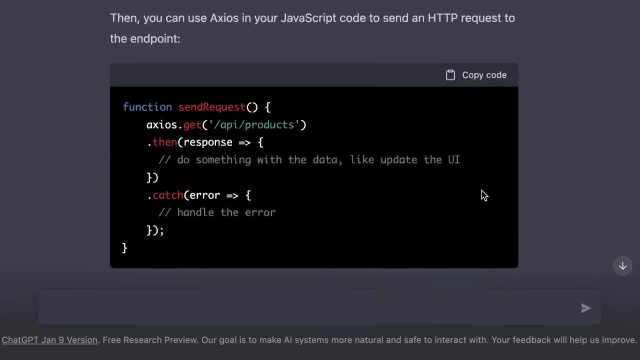 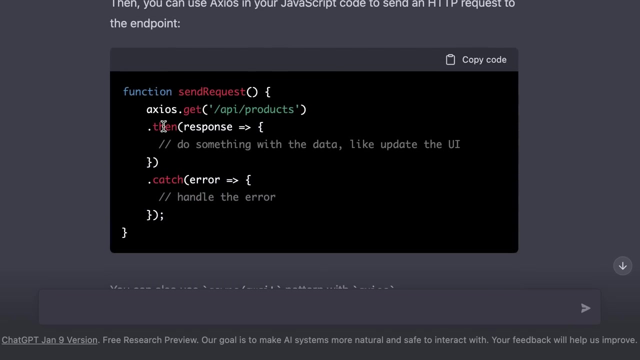 for sending HTTP requests. Now take a look. Alright, now we have the instructions for installing Axios using NPM or yarn, as well as a modified example using Axios Beautiful. We can also ask chat GPT to help us with compile time or run time errors. Here is an example. 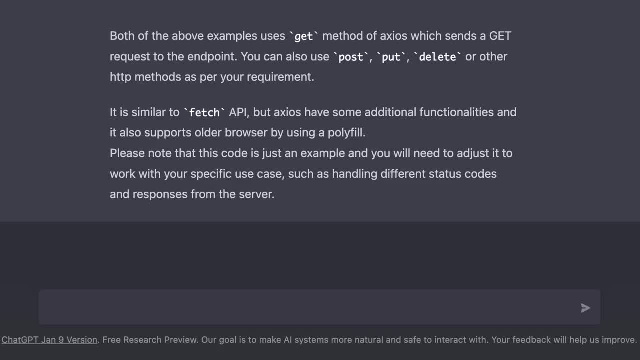 Let's say, as part of writing some JavaScript code, we got an error saying uncaught type error cannot read property, let's say bar of undefined. Anyone who has written a little bit of JavaScript code has probably come across this error, So we can. 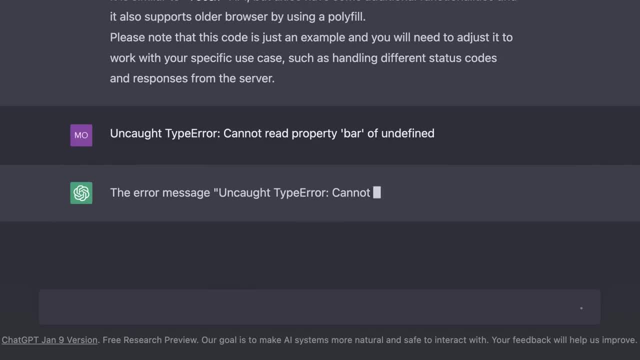 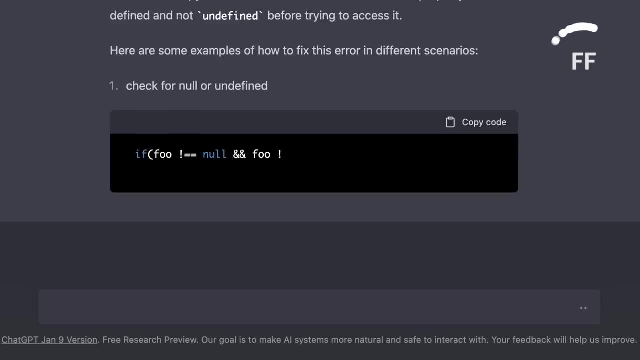 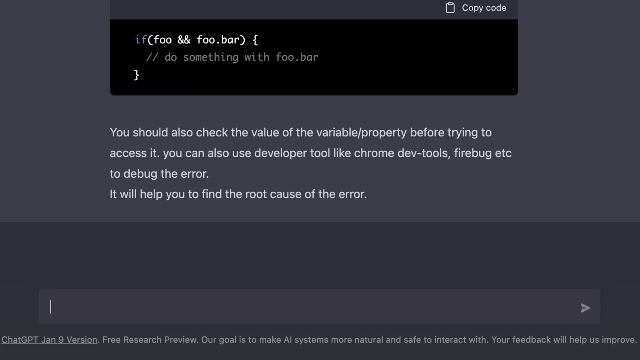 copy paste the error message here. Now chat GPT explains exactly what this error is and how we can potentially solve it. So, going forward, I think a lot of people will start to use chat GPT instead of Google. Now we can also throw react here. 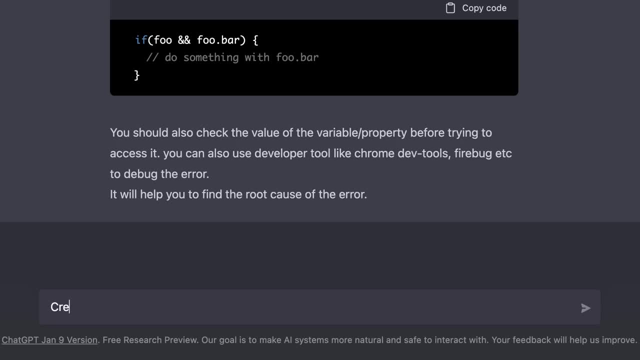 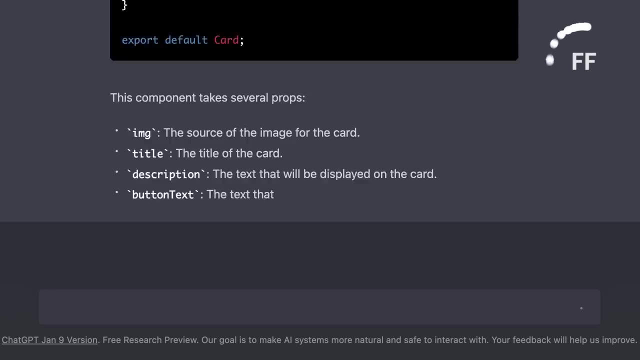 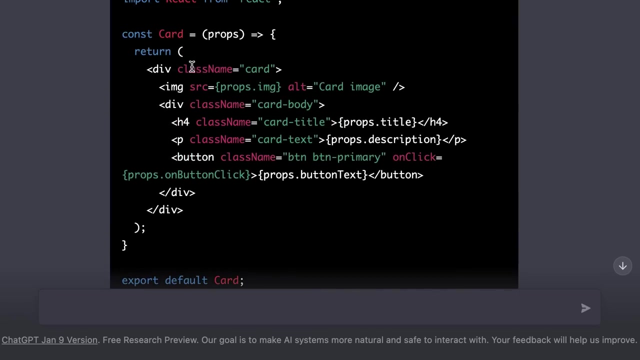 and make the example more interesting. So we can say: create a react component for displaying a card. Alright, let's see what we can do here. Alright, let's see what's happening here. So up here we have an example of a function component for displaying a card. 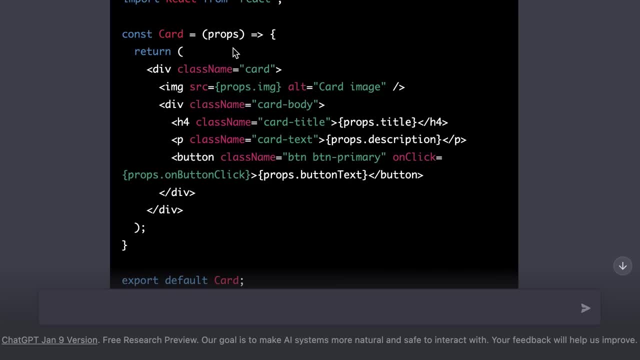 now. I personally don't like to have a parameter called props. it would be nicer to destructure this parameter and grab individual properties like title, description and so on. If you're not familiar with this concept, don't worry, just continue watching. we're not going to do a lot of fancy JavaScript stuff. 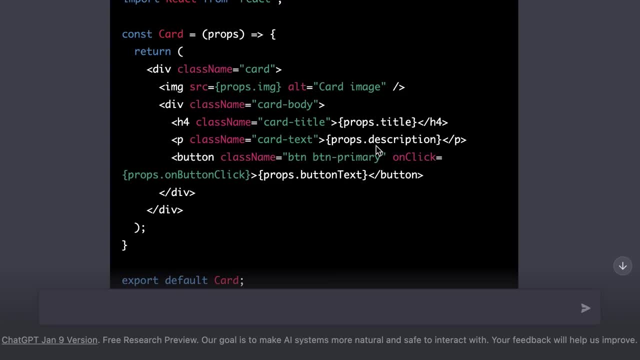 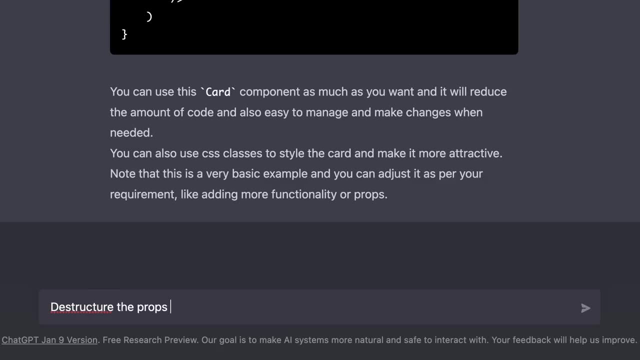 in this video. this is just to open your eyes to the possibilities. So let's take this to the next level and say, destructure the props parameter. So the beautiful thing about chat GPT is that it remembers our conversations. So let's go ahead. 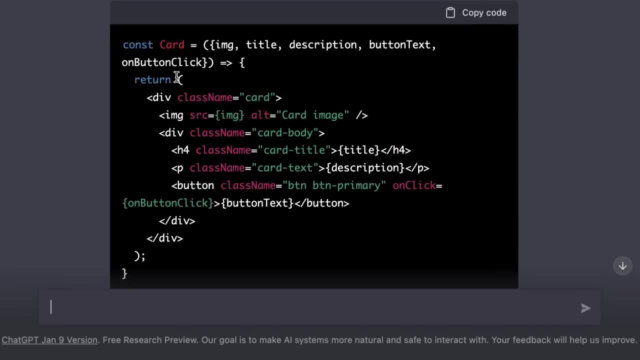 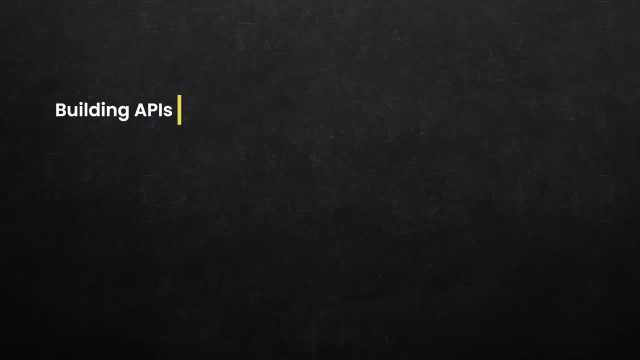 alright, now we have a new implementation of the card component, with the props parameter destructured. Alright, now let's move on and look at a few examples involving backend development. For example, we can ask chat GPT to build an API for us with node and. 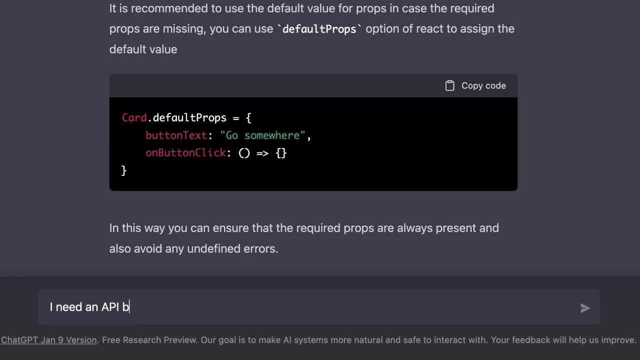 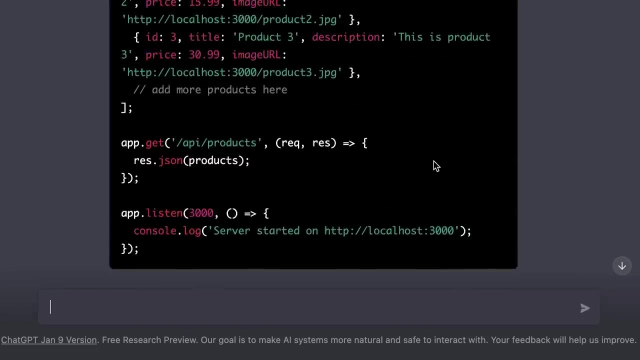 express. So here we can say: I need an API built with expressjs to return the list of products. Each product should have attributes like id, title, description, price and image url. Alright, look at this implementation. In this implementation we have: 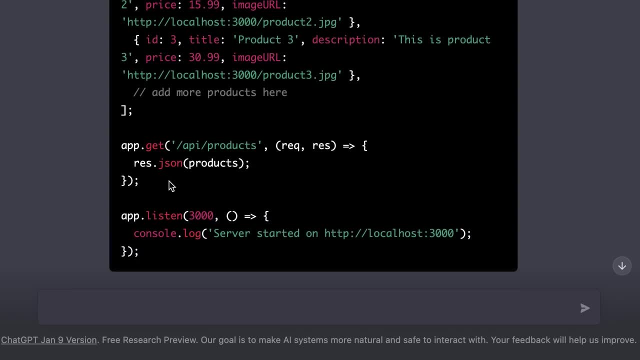 an area of products stored in memory and we have an API endpoint exposed at this url. I don't want to have an area of products in memory. I want this products to be stored in a mongodb database. So here we can say: modify the code and retrieve. 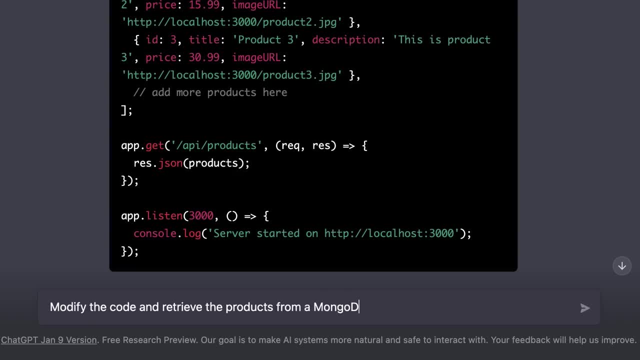 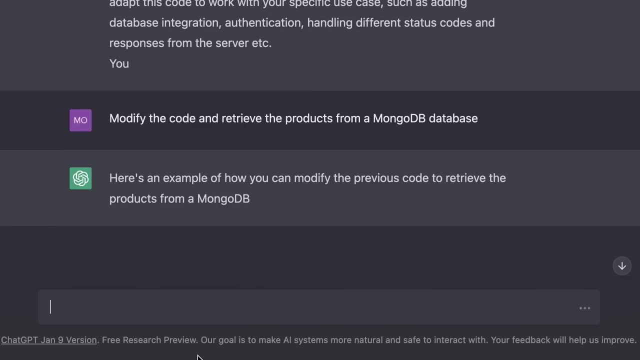 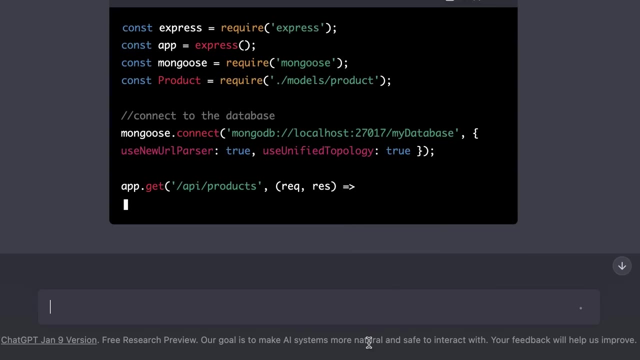 the products from a mongodb or a mysql or a postgres- whatever- database. Now we get a new implementation where products are retrieved from a mongodb database using the mongoose library. Here it is Now, in this implementation, the type of these parameters is not clear. 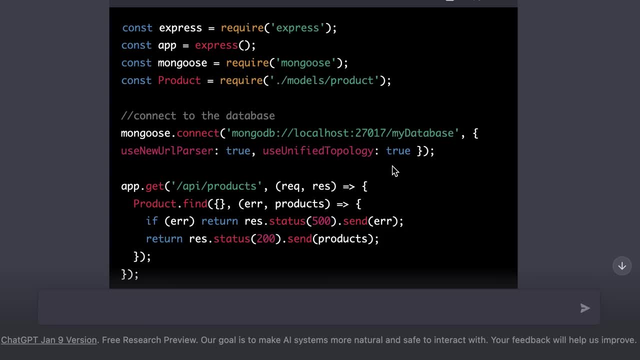 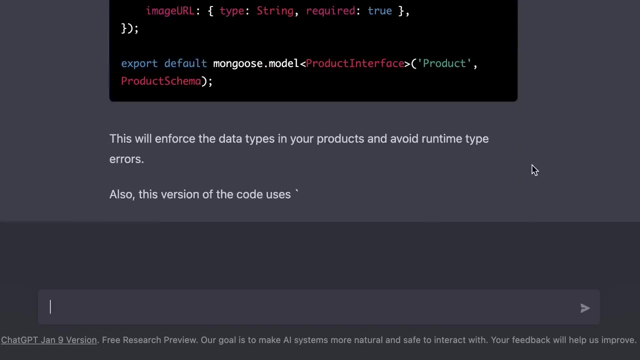 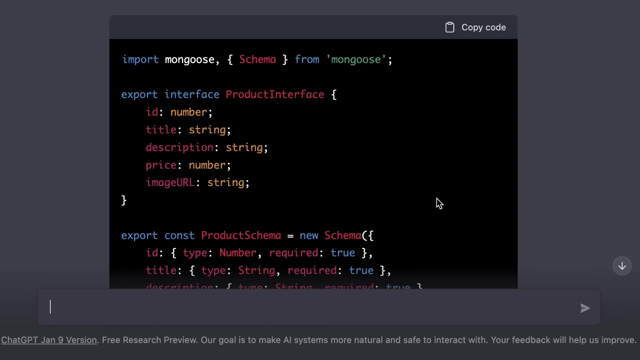 because this code is just plain javascript. Now we can improve this implementation and use typescript. So we can say: use typescript in this code. Now we have a new implementation of the same web server, implemented using typescript. Now, let's say, you're a python developer, you don't want to use javascript. 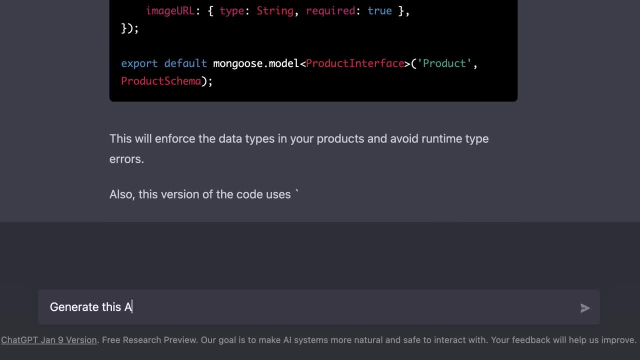 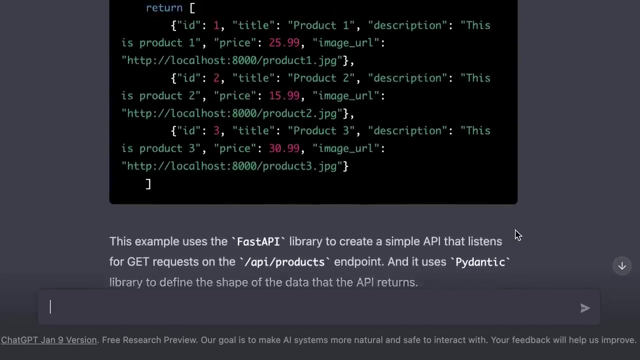 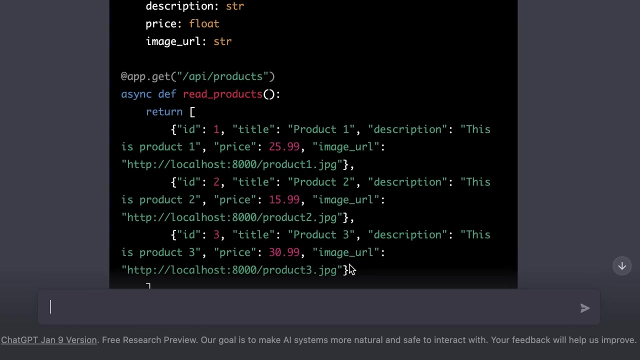 So here we can say: generate this API using python and fastAPI, which is another library for building APIs using python. So all right, now we have a new implementation, but in this implementation our products are stored in memory. again we can talk to chatGPT and customize this further. 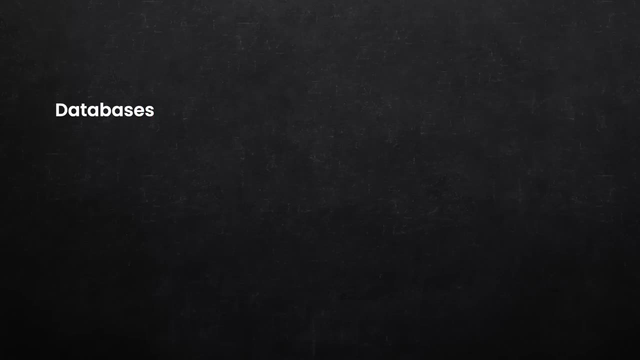 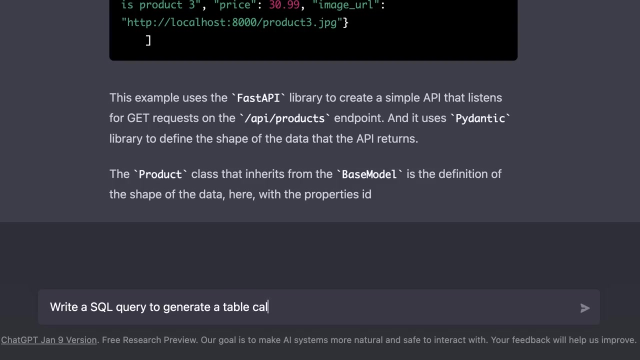 All right, now let's look at a few examples involving databases. This one is pretty interesting. So I'm going to say: write a sql query to generate a table called products with four columns- Note that I'm not specifying the columns, but I'm going to say: write a sql query to generate a table called products with four columns. 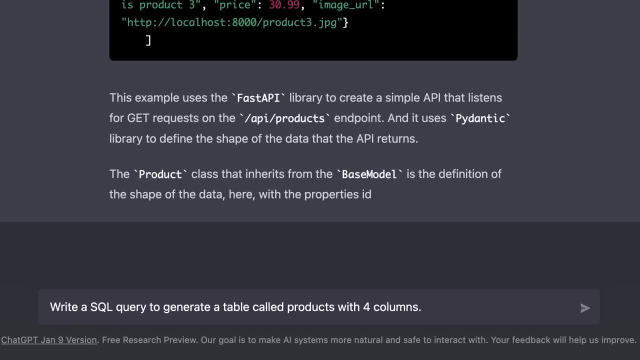 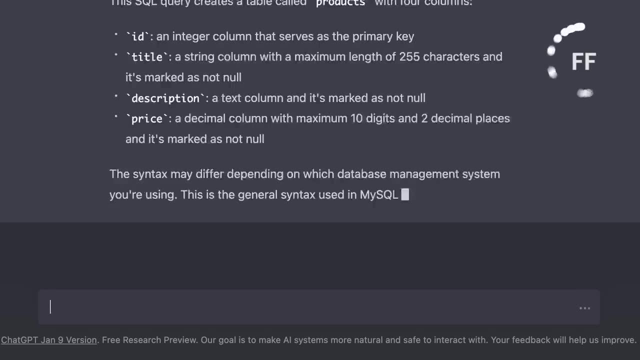 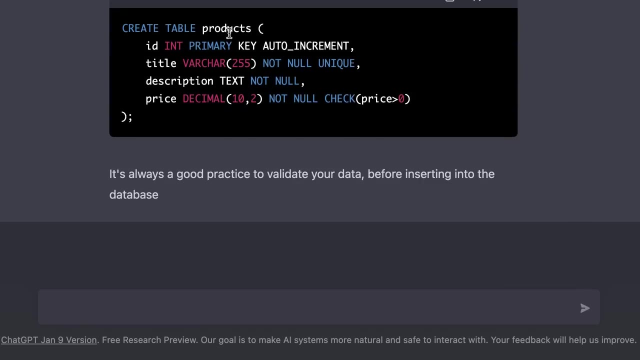 Note that I'm not specifying the columns, names and types here. I'm just saying I want a product table with four columns. See what happens Now. look, chatGPT is smart enough to know that quite often products have attributes like id title. 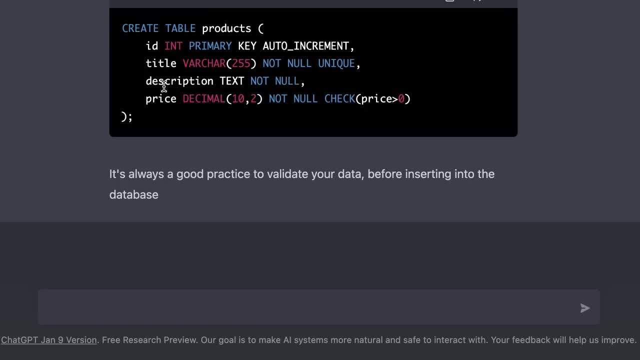 description and price. If this is not what you want, you can always specify the name and type of each column. For example, we can say: write a sql query to generate a table called products with these columns. Now here we press shift and enter, so we go to the next line and on each 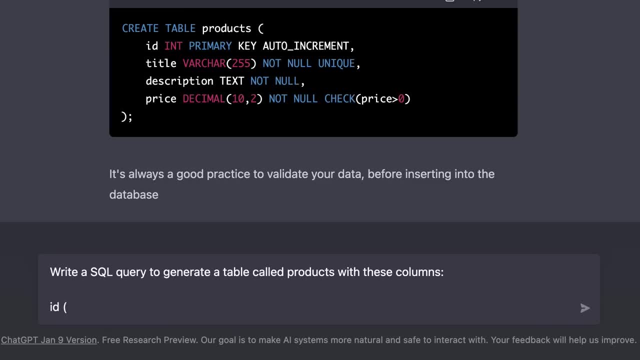 line. we can list a column, We can say: id of type integer, title of type string, category of type integer, unit, price of type float and image url of type string, And you don't necessarily have to put the type in parenthesis. you can type a colon and right after that 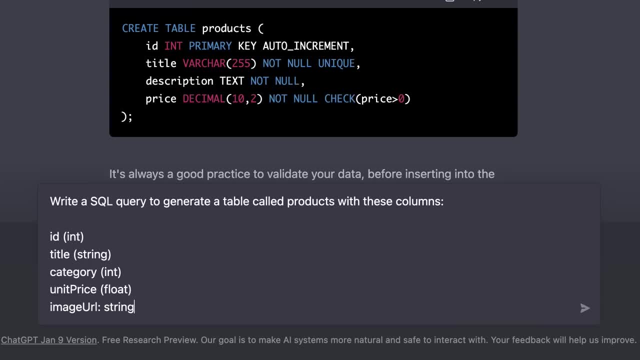 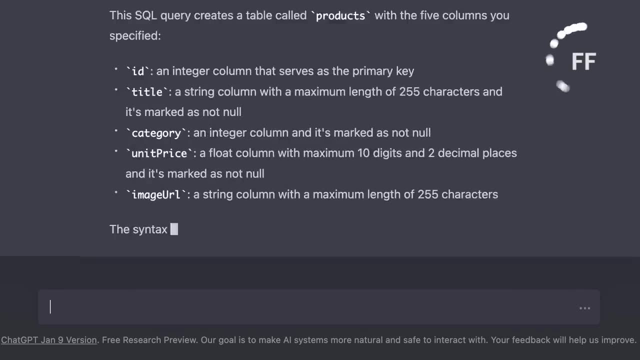 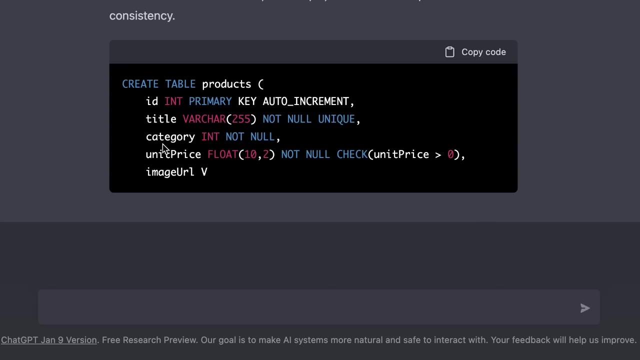 you can specify the type. So chatGPT doesn't have a particular syntax you have to follow, because it can understand human language. Alright, now in the products table we have columns like id, title, category, unit, price and so on. We can also use 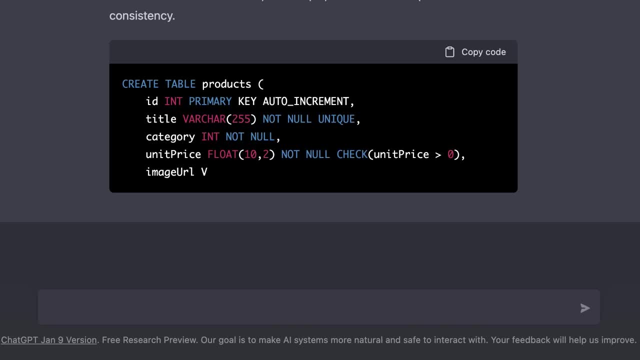 chatGPT to write queries for retrieving or updating data. For example. here we can say: write a query to retrieve the top 5 customers in Manhattan- Note that we don't currently have a table called customers, so we're just asking chatGPT to write a query to retrieve the top 5 customers in. 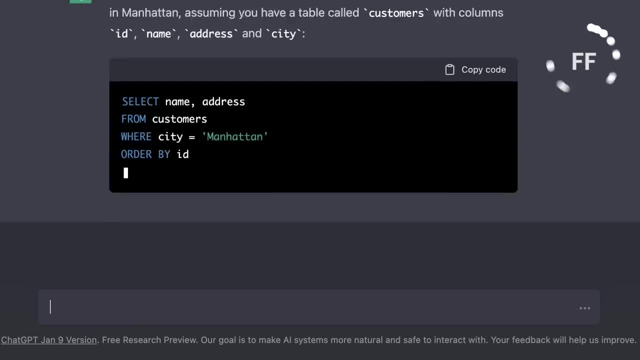 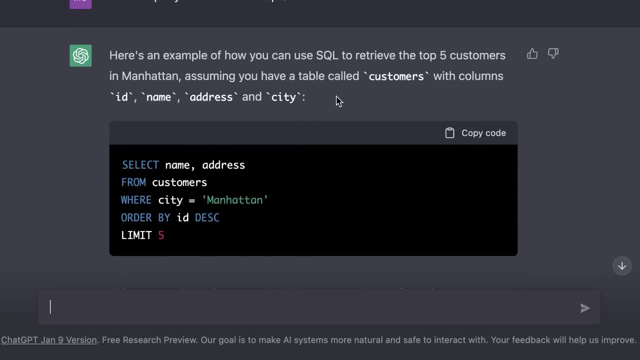 Manhattan. Take a look Alright in this example. chatGPT has assumed that we have a table called customers with these columns: id name, address and city. If our customers table has a different schema, we need to specify that ahead of time. So we specify the name and type. 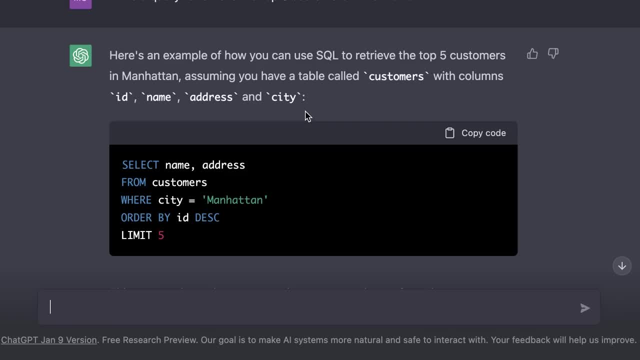 of each column. then we ask chatGPT to write a query to retrieve the top 5 customers. Now look at this query. in this query we're simply selecting customers who are located in Manhattan. So in this query the customers are sorted by their id in descending order. 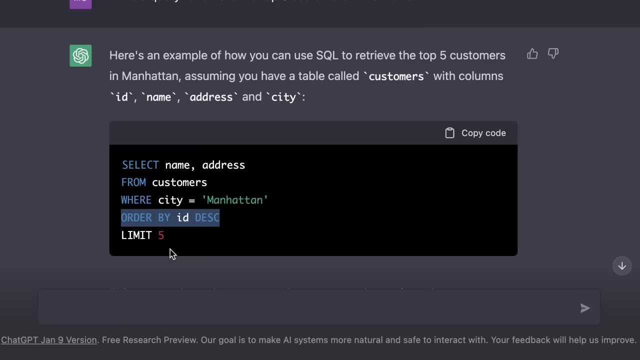 and the top 5 are returned. This is not what we really want. What we want is the top customers who have spent the most. So we need to be more specific with our prompt. So we need to tell chatGPT to do a. 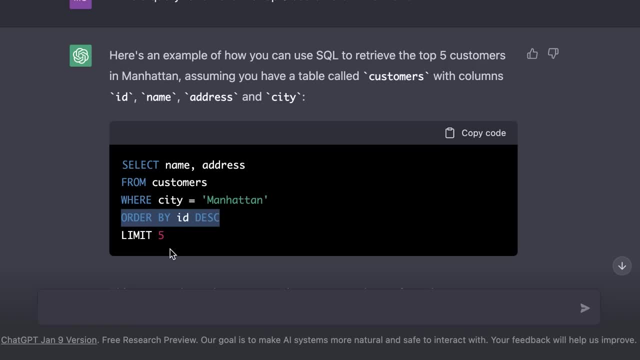 join with the orders table to find out how much each customer has spent. Then it should grab the top 5 customers who have spent the most. So we can say: revise this query and join the customers table with the orders table to find out how much each customer. 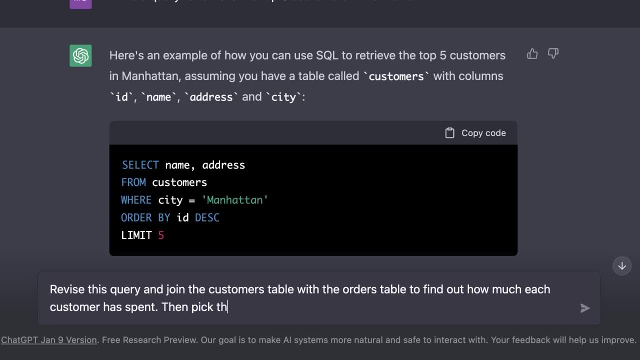 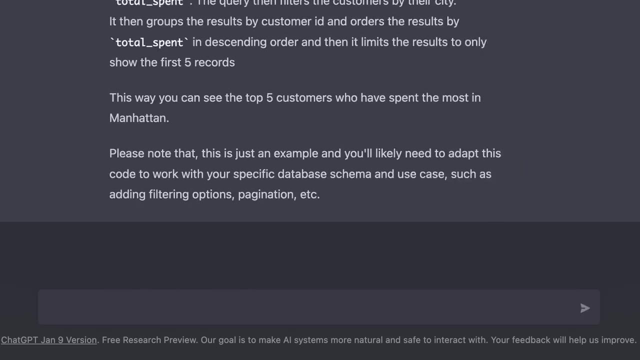 has spent, Then pick the top 5 who have spent the most, And again, here we can specify the schema of the orders table as well. So let's go ahead. alright, look now. chatGPT is assuming that we have 2 tables. 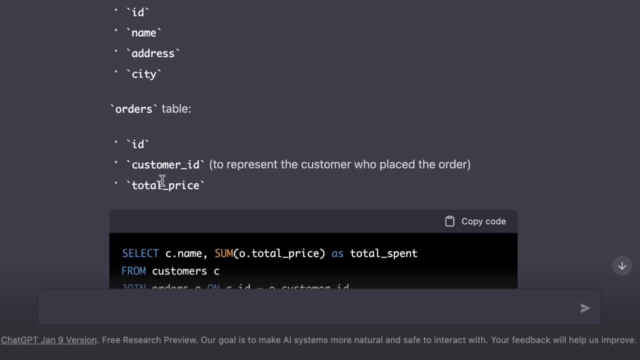 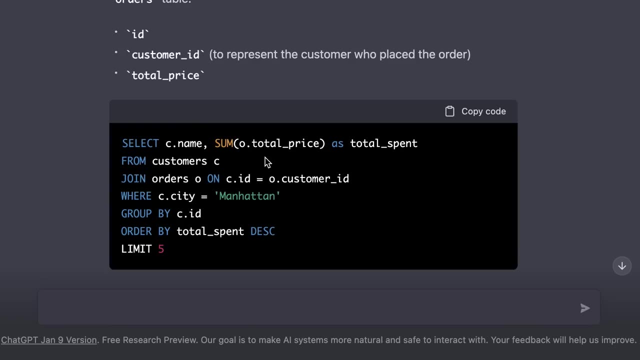 customers with these columns and orders with these other columns and based on this schema, it has revised our query to retrieve the top 5 customers who have spent the most. So that's it, guys. there are endless ways to get creative and use chatGPT. I hope you. 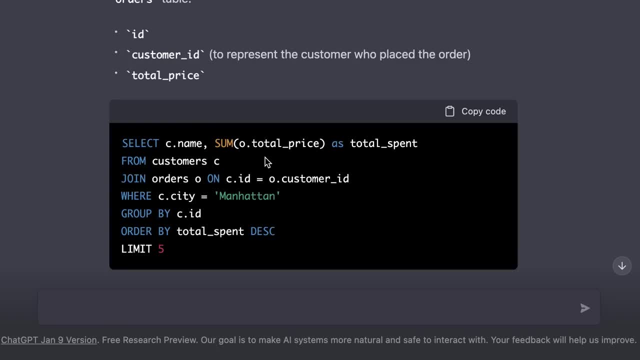 found this video helpful. if you enjoyed it, please give it a like and subscribe for more videos like this. Also, let me know in the comment section what interesting questions you have asked, chatGPT. I would love to hear from you. So thanks for watching and I will see you in the next video. 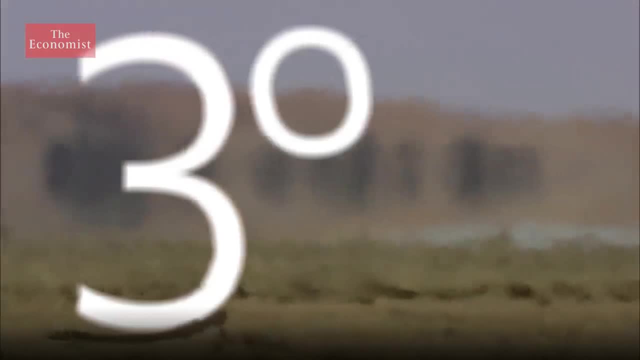 Three degrees. It can be the difference between snow and sleet, wearing a jacket or not. In your day-to-day life, it may not seem significant, but three degrees of global warming would be catastrophic. 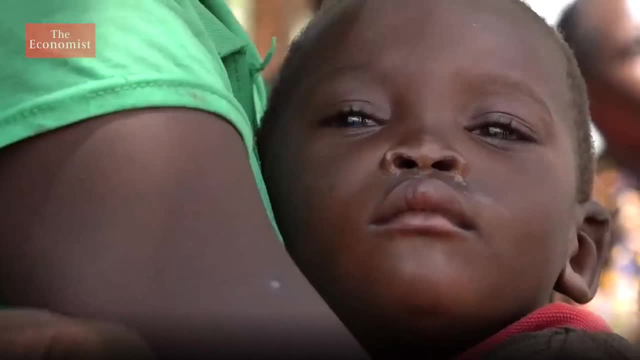 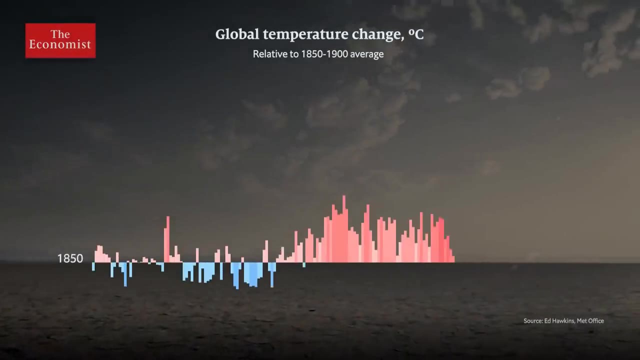 Heatwaves, droughts, extreme precipitation, even fire. Three degrees of warming is really disastrous. The scary thing is, the world is well on its way there. 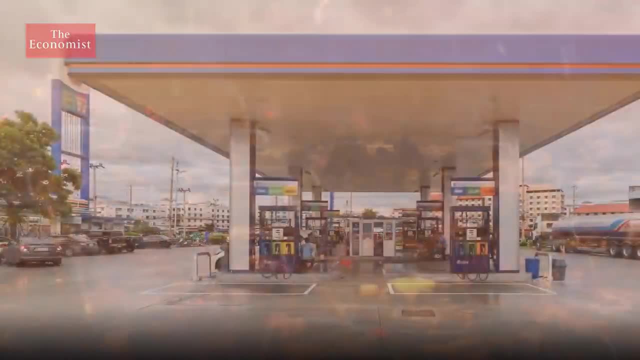 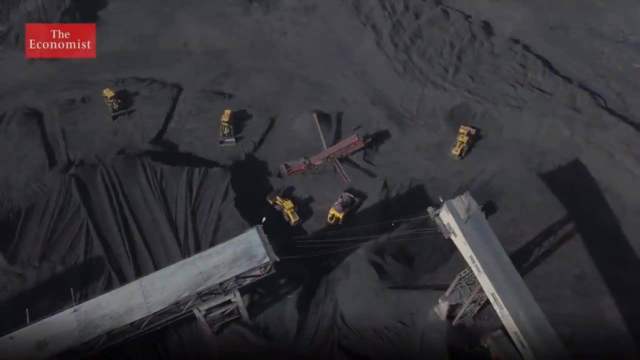 Since the Industrial Revolution, the Earth has warmed between 1.1 and 1.3 degrees Celsius. This is a problem that babies you pass in the street will have to live with. 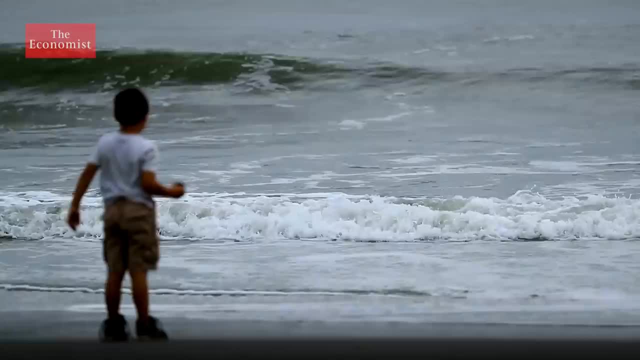 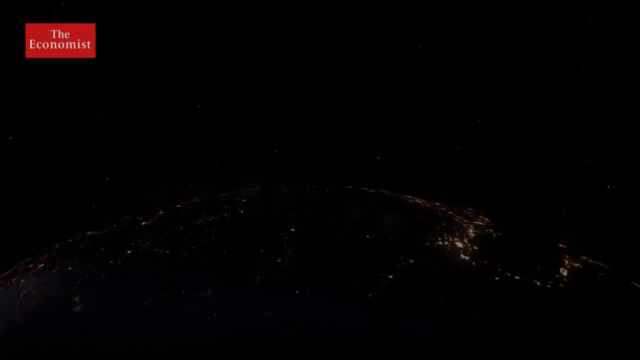 Children born today are up to seven times more likely to face extreme weather than their grandparents. If global temperatures do rise by three degrees, what would their world look like? The world is going to be a mess. 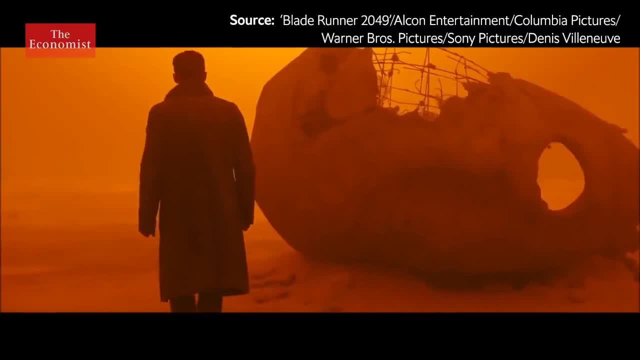 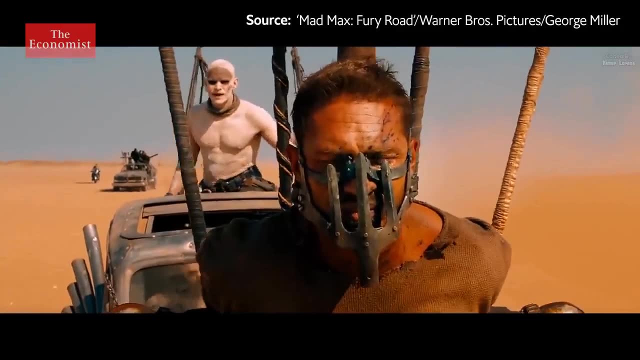 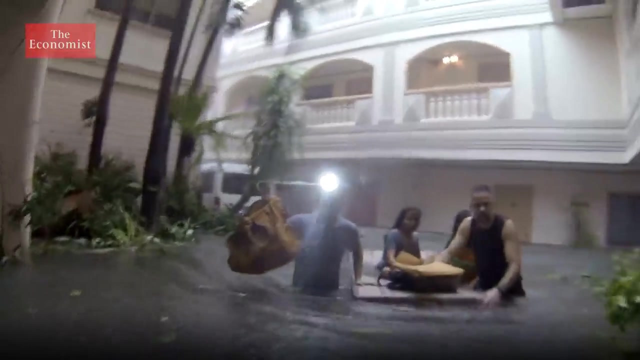 Rising sea levels. Desertification. Hollywood has always enjoyed imagining the end of the world. While blockbusters like this are clearly fiction, this film will show the scenario we all face, unless more drastic measures are taken to stop burning fossil fuels. 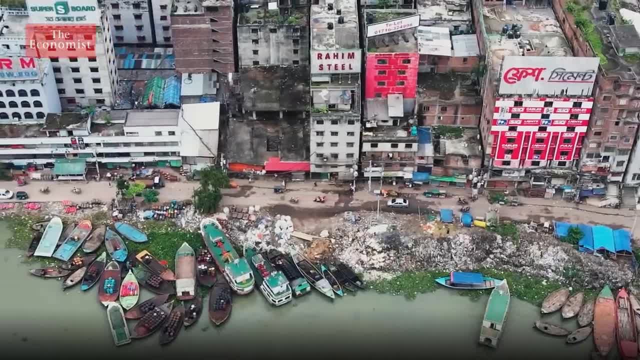 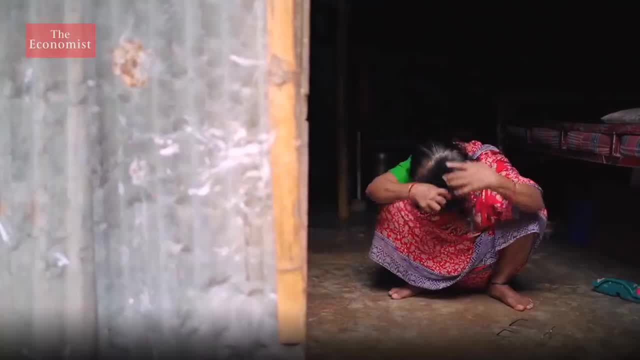 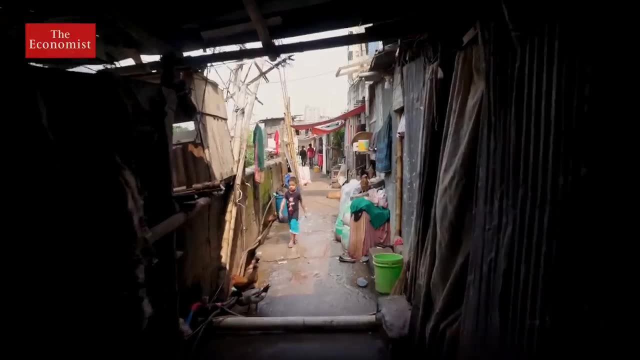 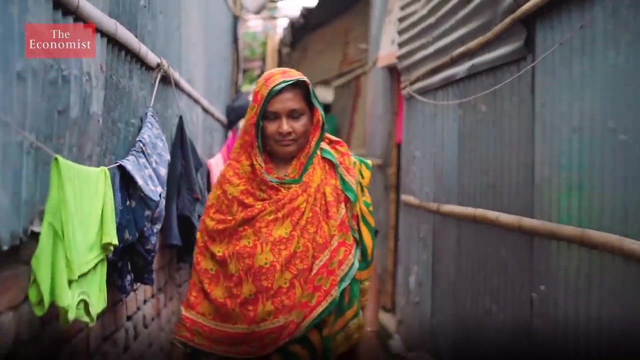 In some parts of the world, the effects of inaction are already clear. The slums of Bangladesh's capital are filling up with climate migrants. Minara comes from Bola district, an area in southern Bangladesh. There, like many other parts of the country, rivers swollen by heavier rain and melting Himalayan glaciers are washing away people's homes. Many, like her, have lost everything.